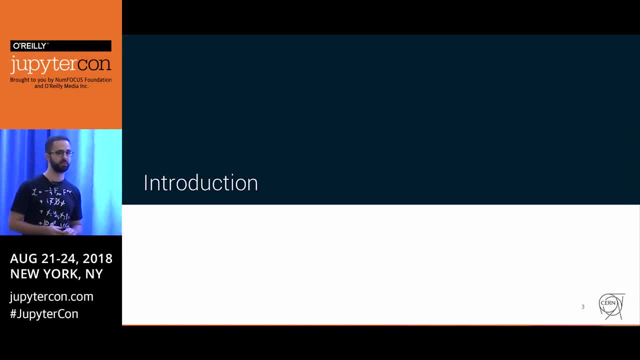 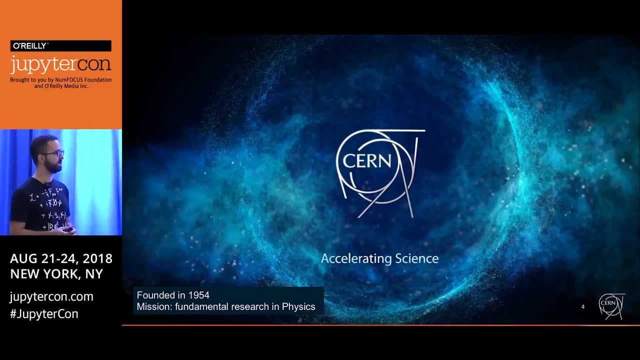 But let's start with the context and explain to you what CERN is. CERN is a physics laboratory- It was founded in 1954, and it's focused on research, technology, education- all of these in the domain of fundamental physics. And probably when I mentioned the words- yes, the word CERN- you thought about this. 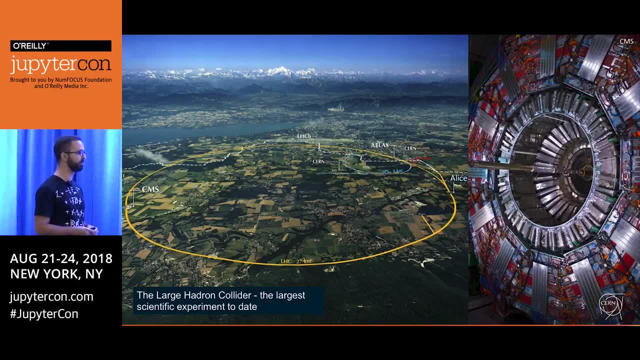 We are home to the largest and the most powerful particle accelerator in the world. It's called Large Hadron Collider, or LHC for short, and it's a ring with 27 kilometers, or almost 17 miles. And why is it useful? 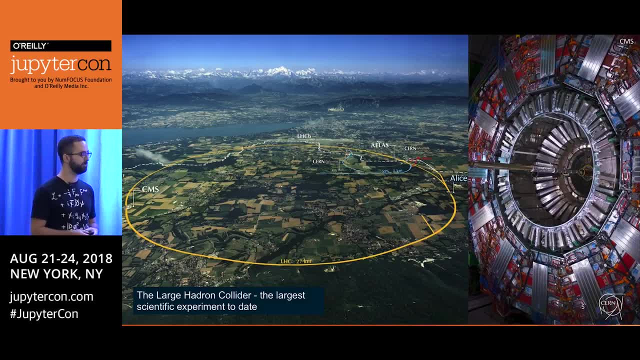 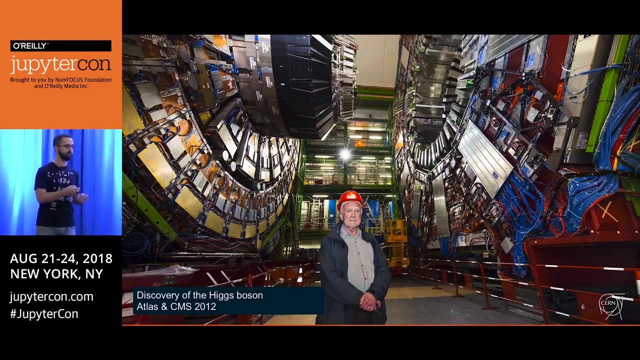 It's useful because it is helping us discover more about the basic building blocks of matter and forces that govern our universe, And it was thanks to it that we discovered the Higgs boson, And, like it, CERN has many other accomplishments in physics. 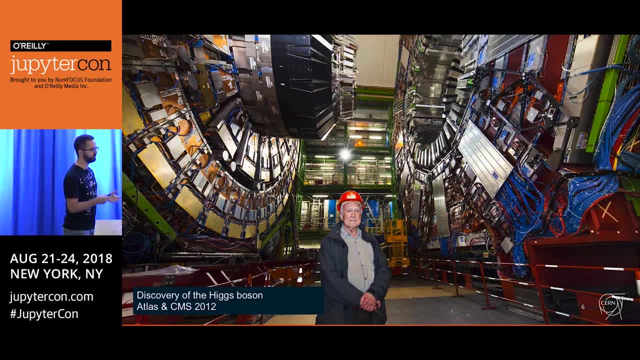 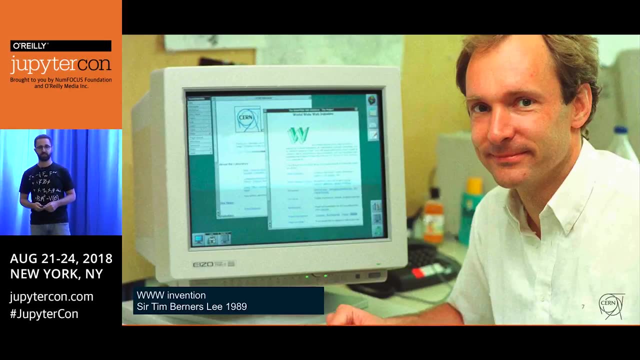 But what I'd like to tell you today is that we not only have a accomplishments in physics. A lot of innovation that comes out of CERN spans multiple areas, And one that I thought is interesting for this audience- and actually it was mentioned this morning- 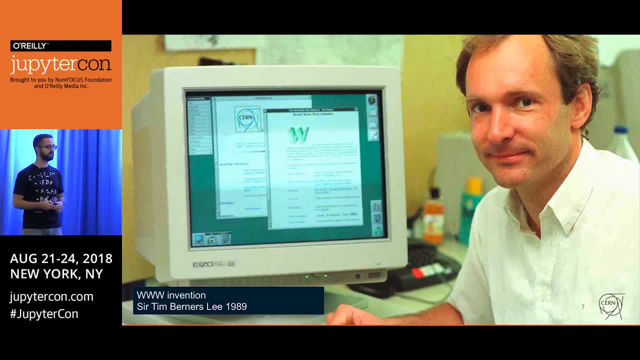 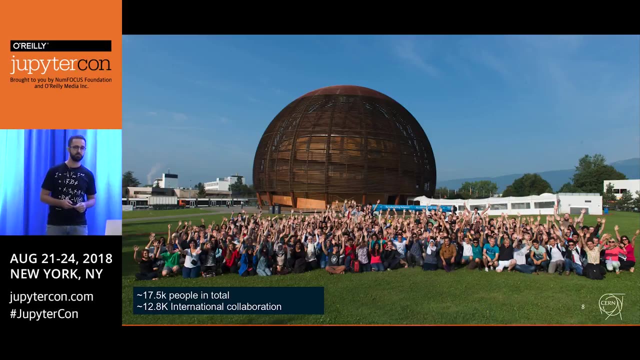 is the invention of web. Sir Tim Berners-Lee was working at CERN when he invented the web, and it's something that now makes Jupyter possible And, like him before, we are a community nowadays of almost 18,000 people working at CERN. 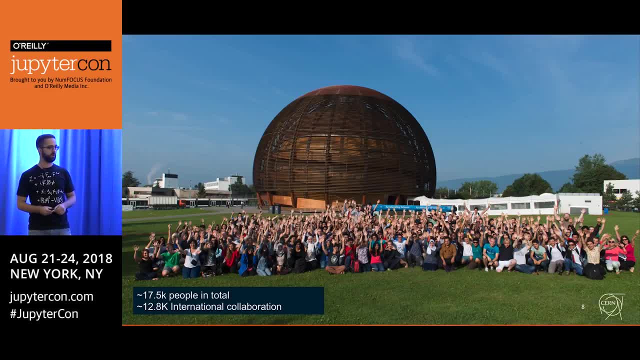 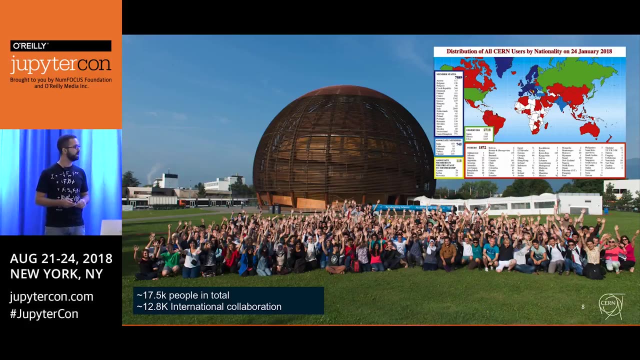 or collaborating with CERN. Out of these 18,000, almost 13,000 are international collaborations. But more than speaking about numbers, it's important also to mention where they are coming from. which countries take part in this massive experiment? 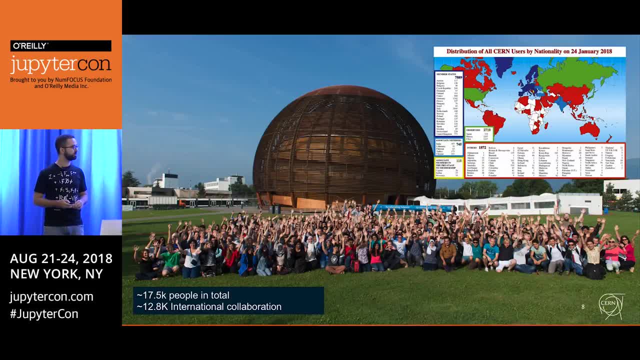 And, as you can see, almost all countries in the world take part with us in the pursuit of new discoveries, And one community very important to us at CERN is the HEP community, or high energy physics community, And this is how they work. 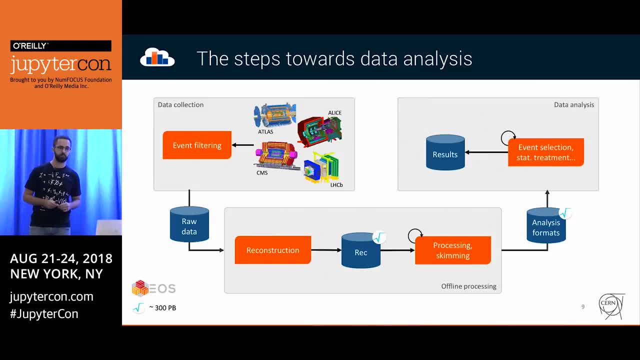 This is their pipeline. To give you some context, at the ALHC we have four main experiments. They are called ATLAS, ALIS, CMS and HEP, And these experiments produce something around one petabyte of raw data per second. 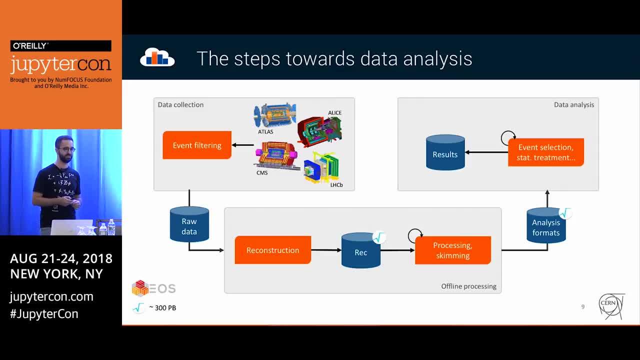 But not all of this data is relevant, and it's such a large amount of data that only a few of this data is really stored, because we do event filtering right out of the detectors, both by hardware and by data, And only then we store this data in our storage system. 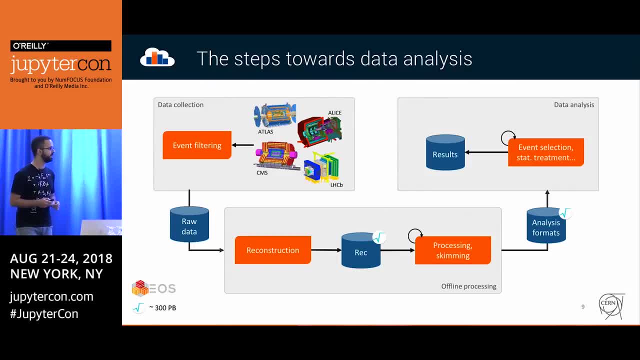 which is called EOS. I will mention a bit about it later- And then it goes through all this pipeline. It gets reconstructed, It's stored in what we call root files. I'm also going to mention what root is in a bit. It gets processed, skimmed and in the end we have 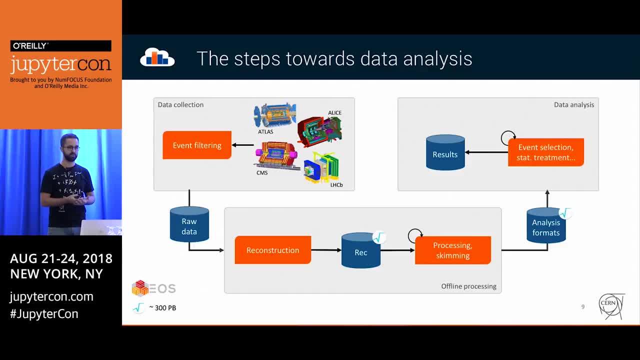 what we call analysis data sets. So these are much smaller data sets, so small that many of our users download them into their own computers and perform the analysis in there And, as you can see and imagine, the last process of the pipeline is the analysis itself. 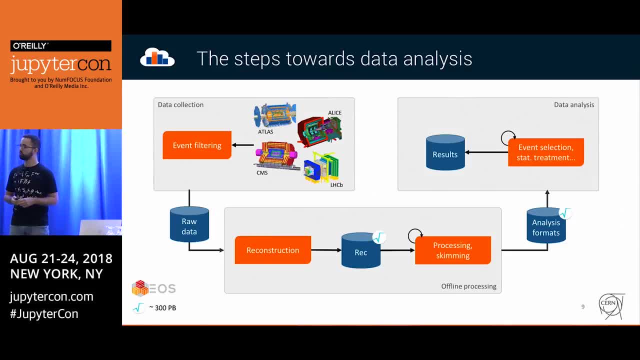 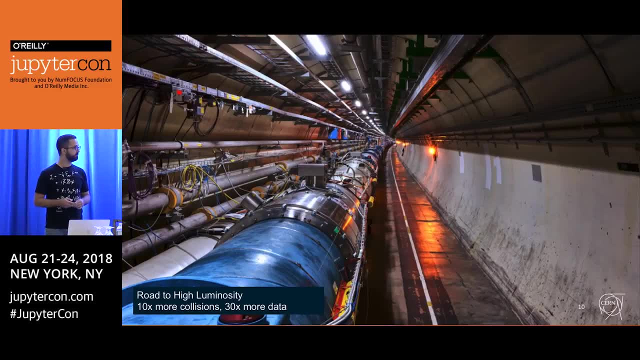 And it's an interactive process, and usually the result is a plot or a graphic. This is something about the future, a challenge that we have, but I decided to mention it right away. The LHC is already at its limits, but we are now building an upgrade to it. 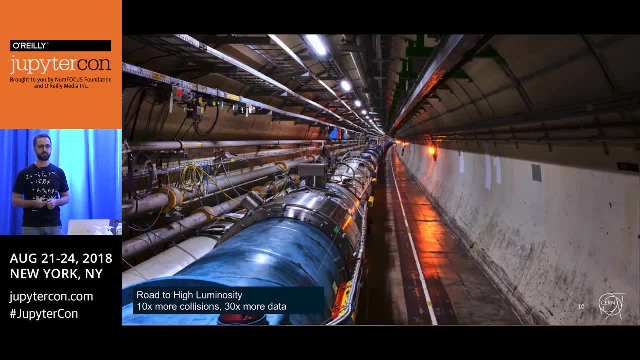 which is called high luminosity, And this upgrade means that we are producing much more collisions in the detectors and it also means that, because we are also improving the resolution of the detectors, we are getting more data and the plan that we, or the information that we have. 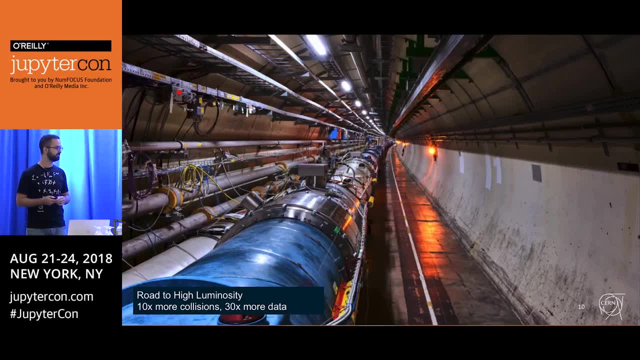 is that almost 13 times more data will be produced at these experiments And, as you can imagine, this is a lot of data And because it's so much, our tools need to get improved and we need to face new challenges to be able to cope with so much data. 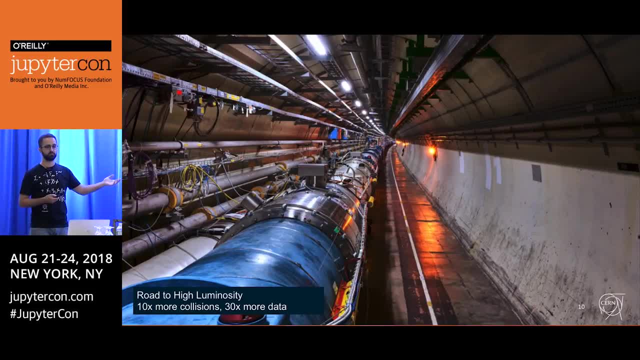 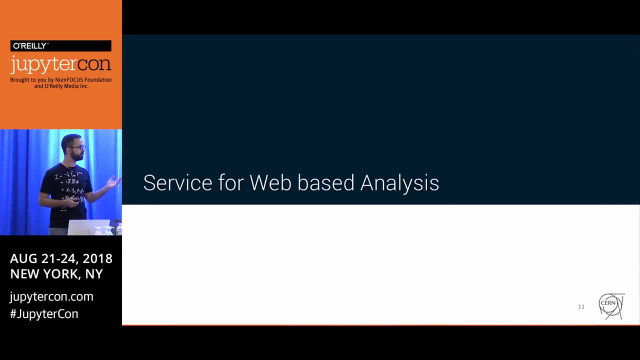 And, for example, I mentioned that many of our researchers download their data set into their computers. Maybe they won't be doing that anymore because it won't fit, So we need to provide tools that will allow them to analyze their data, and SWAN is one of the tools that we think can help. 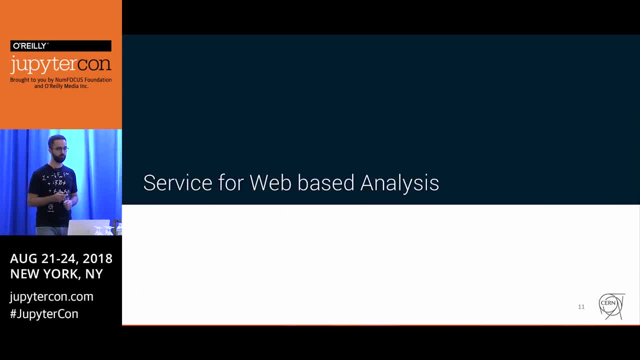 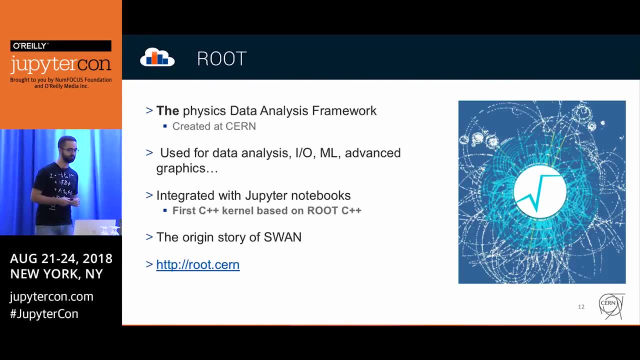 And I'd like to present you now SWAN, but before I'd like to tell you how it came to be, And I already mentioned this name before, and there's a physics data analysis framework at CERN. It was built by us and it's called Root. 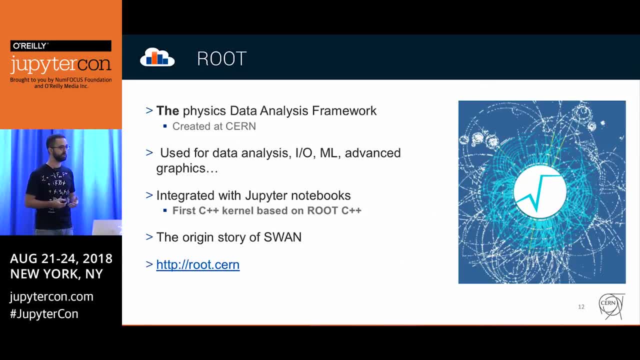 And this is no normal tool, because this is the deep tool that is used by all physicists around the world And it has libraries for whatever you might imagine. It's a very powerful tool and it's spent across all this pipeline of physics research. 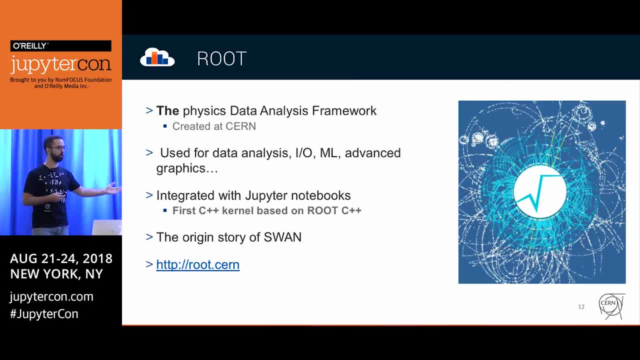 as you mentioned, we store our files in Root formats because we provide such a powerful and optimized libraries for IO. There are many other libraries, but one that might interest this audience is the analysis library that we have, And basically what happened was that. 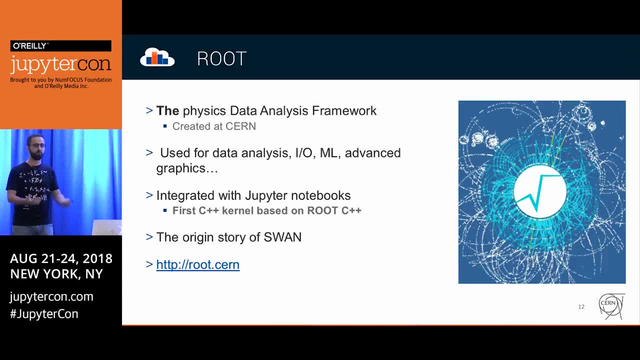 the Root team was thinking: how can we provide an easier way to access this tool? How can our researchers do their analysis in an easier way? And so they thought let's try to make this available as a web service. They looked for tools to integrate with it. 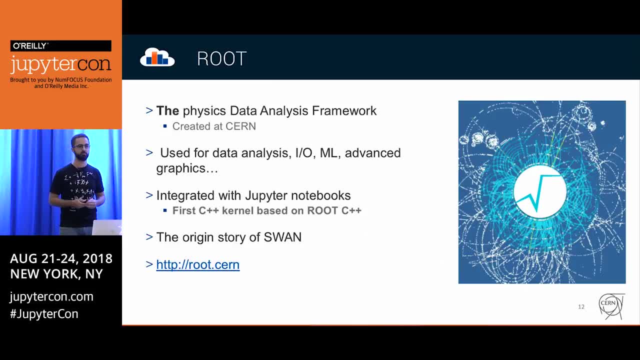 and they found Jupyter. They decided to integrate Jupyter in Root and vice versa, And what happened was that the first C++ kernel that was created to Jupyter was born. So now you have others, other kernels for C++, but the first one came from the Root team. 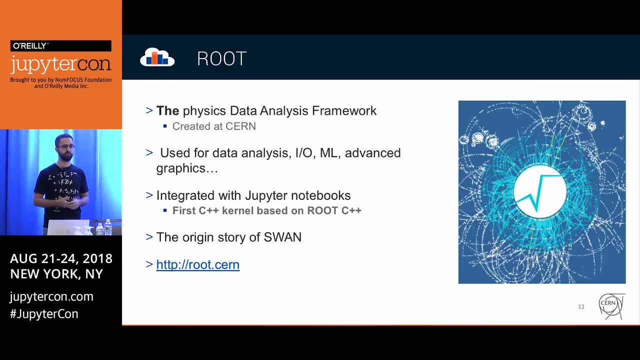 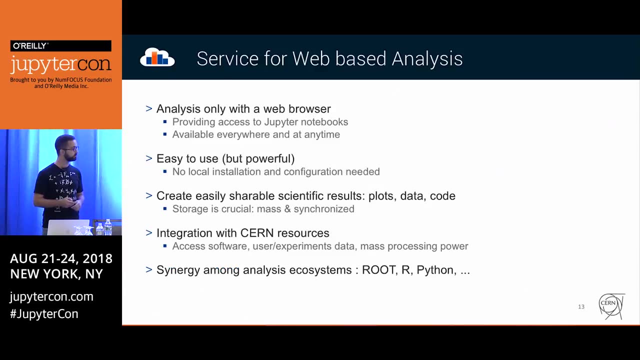 And when the team did this, when they did this integration, they realized maybe we can provide this as a service for our users. So that's what they did three years ago and they created Swan exactly for doing that, And this is what Swan is. 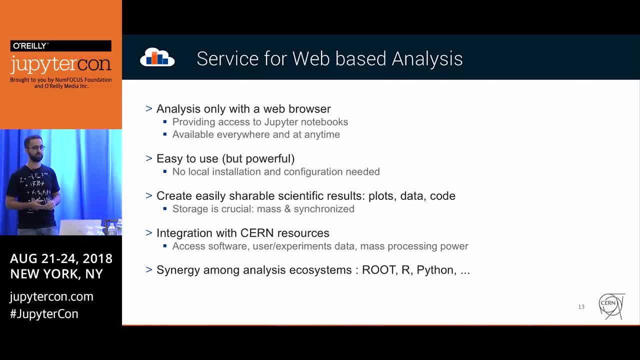 Swan is a service that provides access on demand to notebooks, So it's still powerful. you still have access to the Root framework for analysis, but this time you don't need to install it, you don't need to configure, because everything is available as a web service. 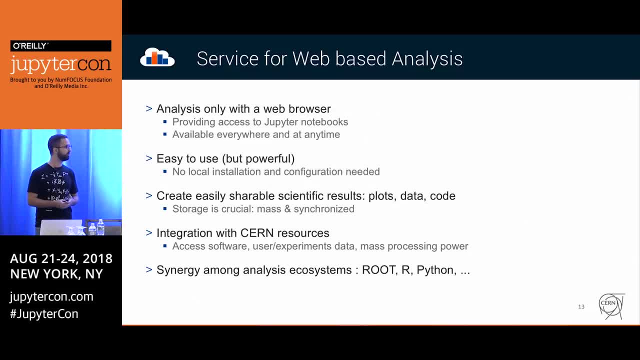 And since Jupyter is such a powerful tool to provide easily shareable scientific results, of course Swan is also a tool for doing the exact same thing, because we are integrating Jupyter. But, as you can imagine, we needed to provide a service. 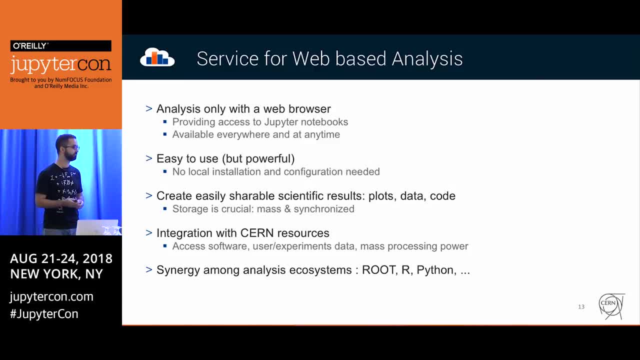 that met our researchers' needs. So we had to integrate a lot of other tools for them to access their software, their data and, of course, all the power that they need to perform their analysis. And although this started as a Root side project, 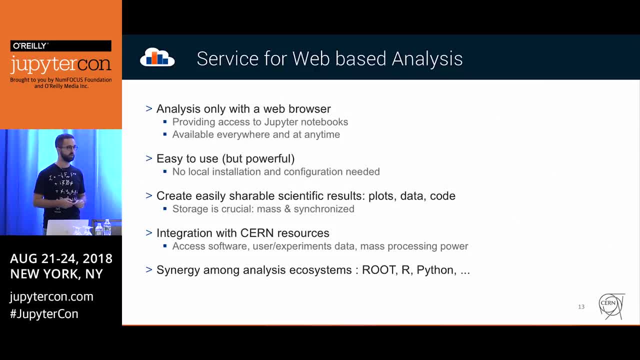 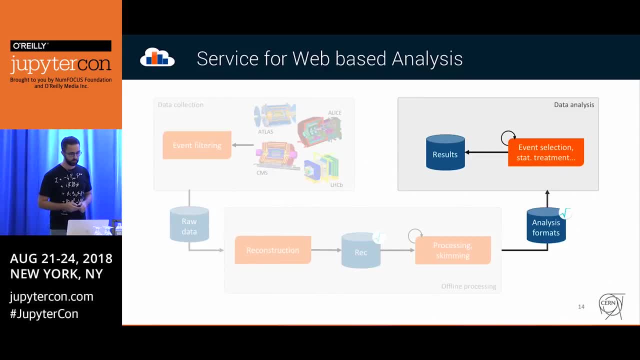 we also integrate with other analysis ecosystems, in our case, the ones that matter to physics, to the HEP community. Getting back to the pipeline, I said that the last step is an interactive step and, as you can imagine, this is the perfect fit for Jupyter. 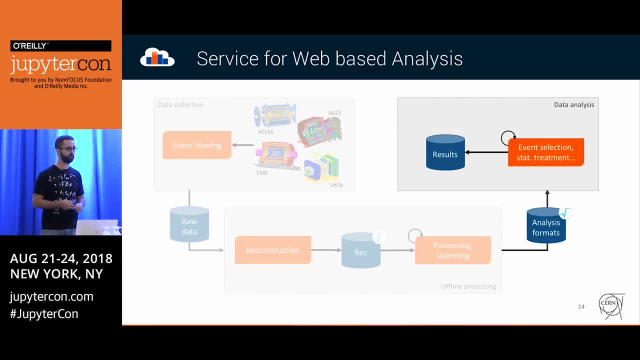 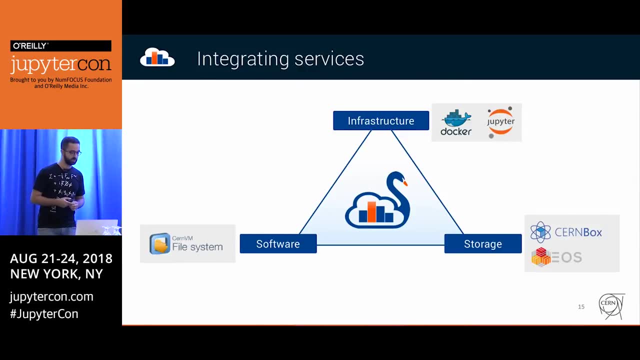 and is actually where it's being used by your community. So they are performing the analysis step with the help of Swan and Jupyter. These are the three pillars of the service. Of course, if we wanted to provide access to software and storage, to data. 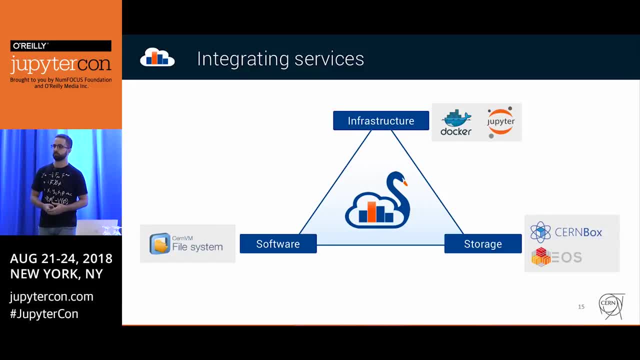 we had to make some choices. We looked around for tools to integrate in the service and what we realized was that we had so much powerful tools in-house, developed at CERN, that were the tools already being used by our community. So there was not a real choice here. 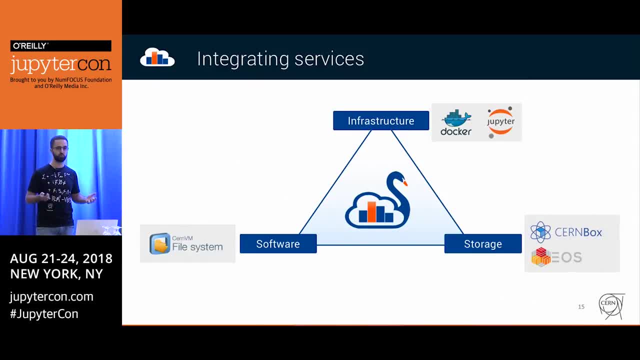 These had to be the tools integrated in the service, And I like to say that Swan is an integrator, not only because it integrates all of these services across multiple departments, but because it's also integrating teams at CERN, And actually the storage team is one of the. 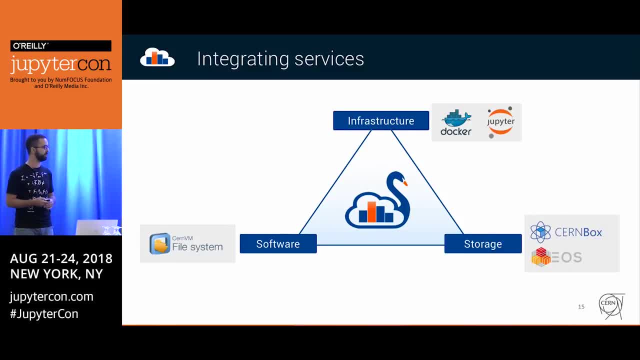 is the team that took part in the project since the beginning, with us And from these three pillars you don't know two of them- storage and software- So I'd like to present them to you. Just a last note here: all of these tools are open source. 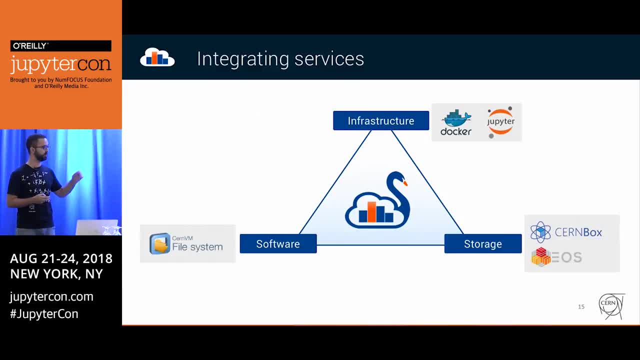 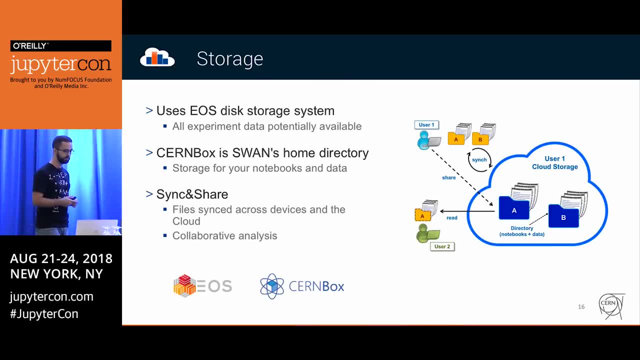 So these are our contribution to the community. So if you want, you might be able to use it in your own deployments. But let's start with storage. I mentioned that in CERN all this data is stored in what we call EOS is our disk storage system. 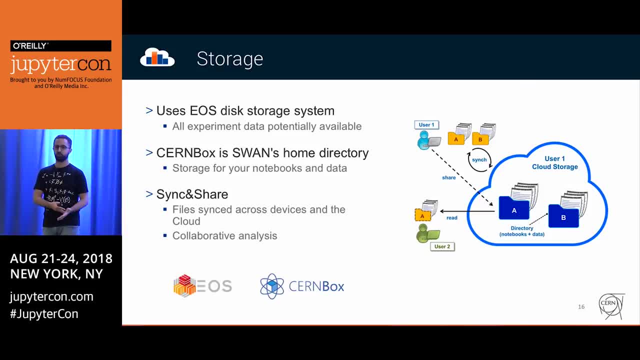 So we decided to integrate it in Swan And by doing so, all of the experiments data is already available to the users once they start their sessions with Jupyter. And one good thing of EOS is that it also provides a user space. So if you have a CERN account, 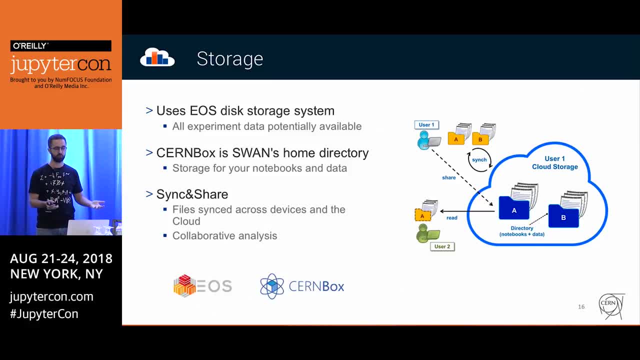 you have a space where you can store all of your files, usually work-related files- And there's a service called CERN Box which allows you to access this storage space, And it's more or less like Dropbox. okay, but it's the one developed at CERN. 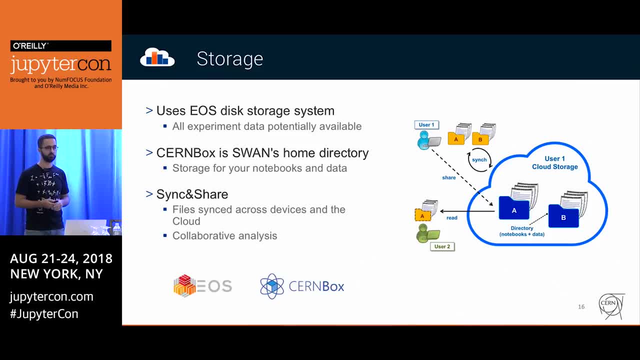 And it allows you to sync all of these files across devices. So you can imagine you can start doing your analysis locally in your computer and then continue in Swan. Everything is synced, You don't have to think much about it, And it also provides. 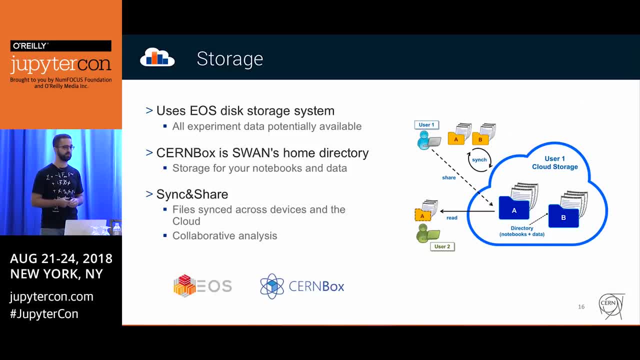 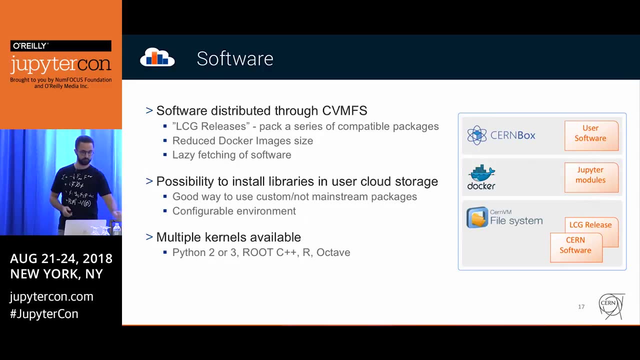 a very interesting functionality that is sharing. Of course, collaborative analysis is very important in our community. Sorry, just a sec. And then there's software Again. we have a tool at CERN called CVMFS. This is a read-only distributed system. 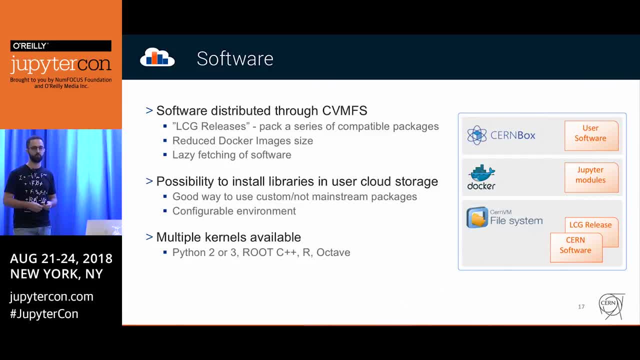 that we use to distribute software across all of our. So this is a read-only distributed system that we use to distribute software across all of our equipment, across our grade, the worldwide grade that we have, the worldwide grade that we have- And inside this system. 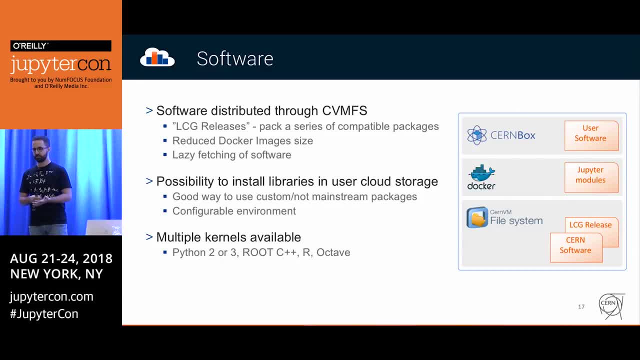 we have what we call LCG Releases. What an LCG Release is is basically a package is basically a package where you put some software libraries, where you put some software libraries with specific versions and we install them, Or the team that builds this system installs them. 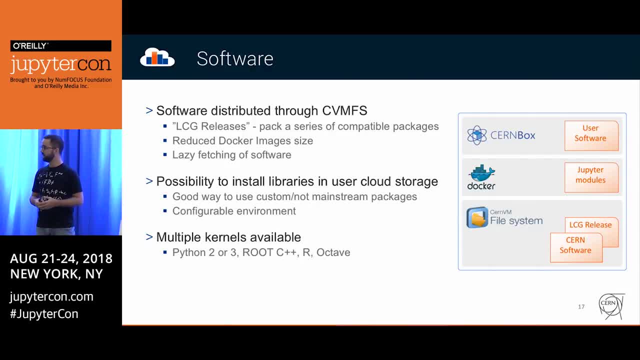 Or the team that builds this system installs them, And they guarantee that all of these packages compatible with each other. so when you select an LCG release, when you're starting your session, you get all of these hundreds of packages that come along. these are the packages that our researchers are using. so by doing so, we 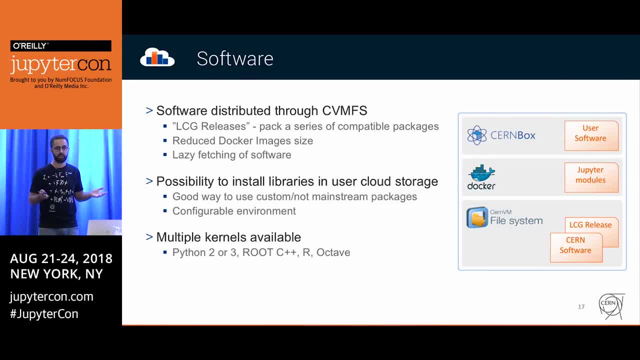 already gave all the software that they need without having to think much about it, and this also allowed us to reduce the docker images that we use, because we are using docker for users and you can imagine that hundreds of packages will produce gigantic docker images, but we don't need to do it because they came. 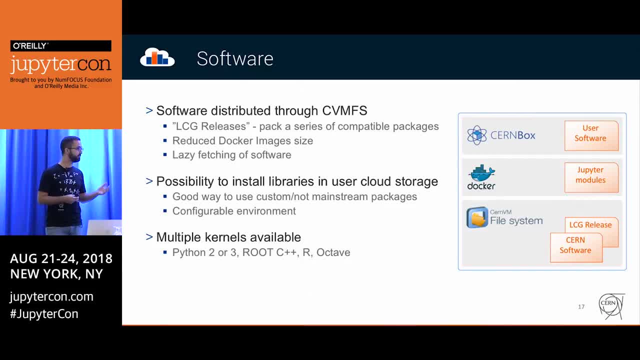 they come from this service, and it's important to mention that this is a lazy service. so if you need only package A and B, you only get back package A and B, even though the stack has hundreds of packages. but of course we have a lot of caching mechanisms to guarantee. 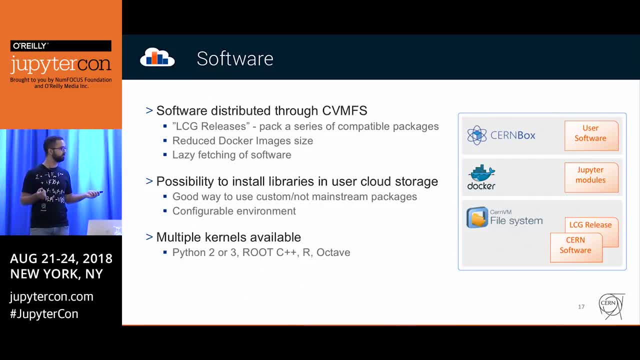 that this works well, and so by doing this, we are providing almost all the packages that our researchers need. but we have multiple users- power users- that need personalization. they need other packages that are not available, so of course, we provide a way for them to install these packages they can. 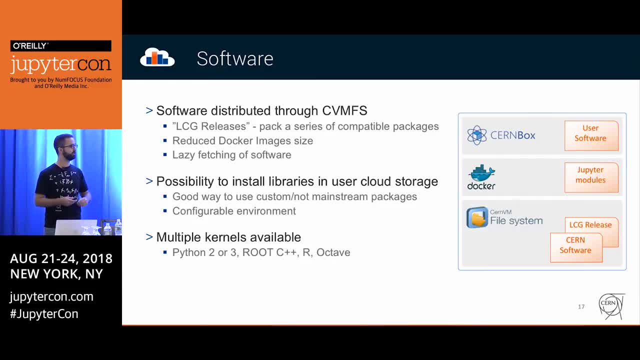 configure all of their environments they call. when they install this situation packages, they get installed inside certain box, so you even get this sync automatically for you, so you still can personalize all of this environment to your needs. and a note: here we are providing four kernels to our users. 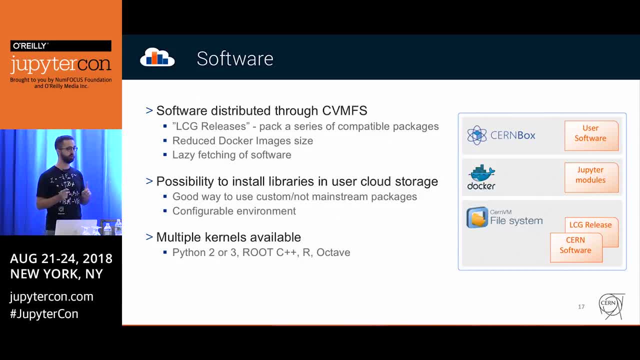 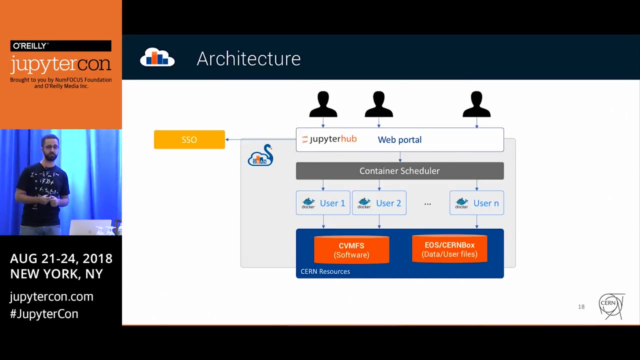 Python in version two or three, depending on the stack that you choose. we have also root C++. of course, this was the origin of this project. then we have R and octave. all of these came come from CVMFS, because that's where we install them. this is the architecture of the service. just so that you know that we 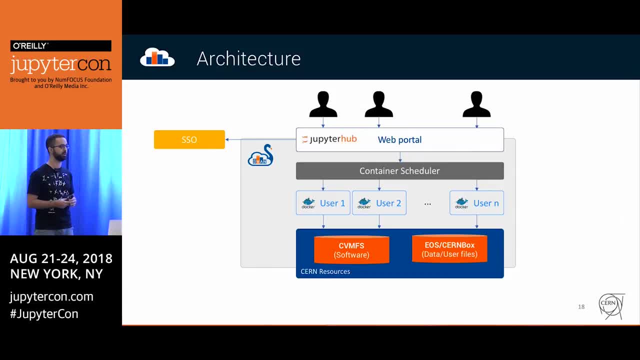 are using Jupyter hub and we are using docker to start user sessions and, of course, we need to integrate with the authentication service at CERN. everything needs to be behind you, our SSO, for security reasons, and we provide all of these access to the, to the infrastructure that I already mentioned, and so we provided the service. 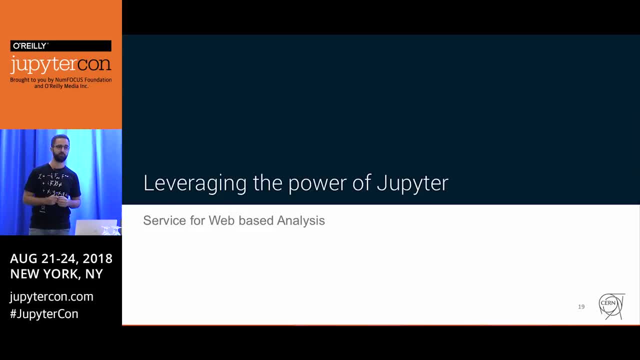 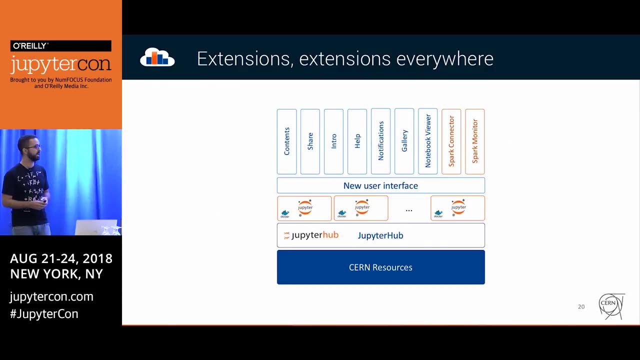 like this: we put Jupyter on top of the infrastructure. but then, of course, we thought we can go further and we can provide more functionality to our users, and so we started by providing a new interface to them, and we put on top a couple of extensions to 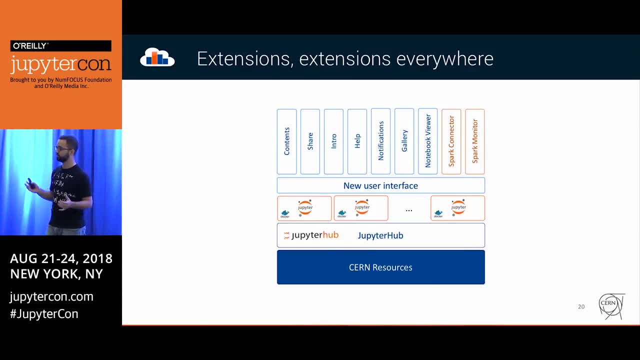 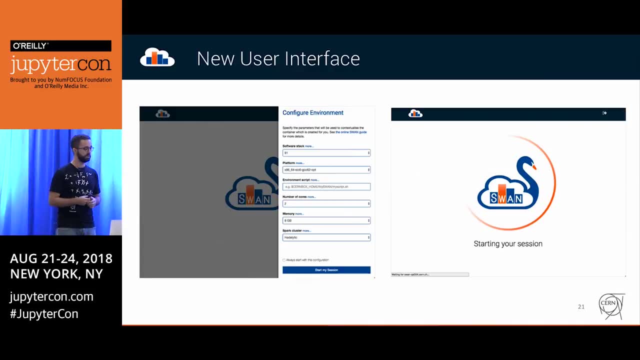 give more functionalities and we have all kinds of extensions. we have NB extensions, server extensions and even kernel extensions. this is how it looks like. so in Jupyter hub, the menu that you can, where you need to start your session, you can select the software stack, so the CVMFS. 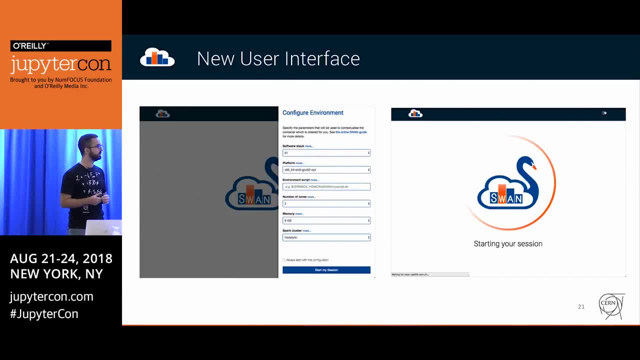 that I mentioned. you choose it here. you can also provide a startup script so you can do whatever you like to your session before Jupyter starts. and there are other options, of course, but one interesting is that our users didn't didn't like to have to do multiple clicks, so we provided them an easy way for them to. 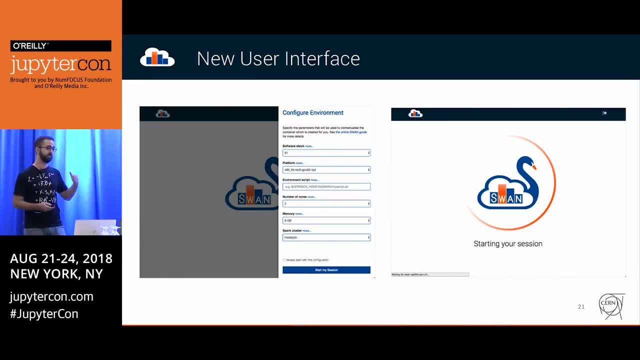 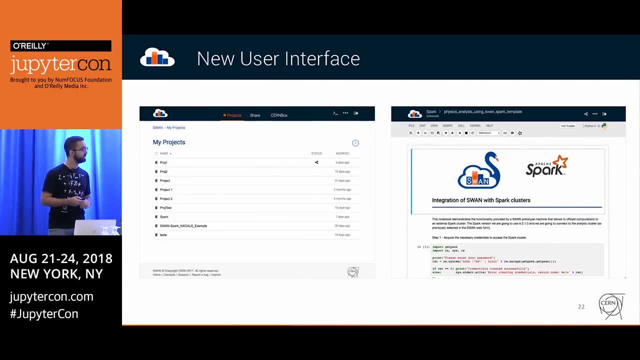 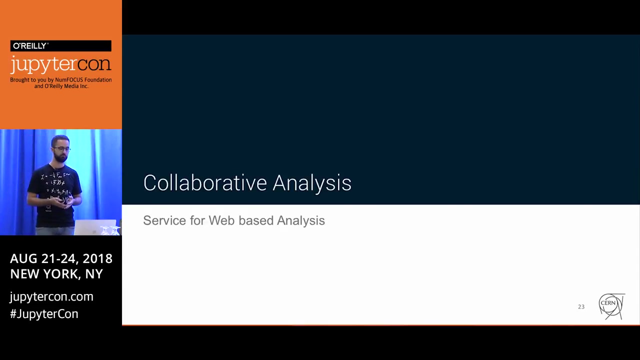 start automatically with the default configuration or the previous selected configuration. so that's what the little checkbox in the end is- again how it looks like. so if you're familiar with Jupyter, you will recognize this. but all of this personalization had a purpose. as I mentioned, collaborative analysis is. 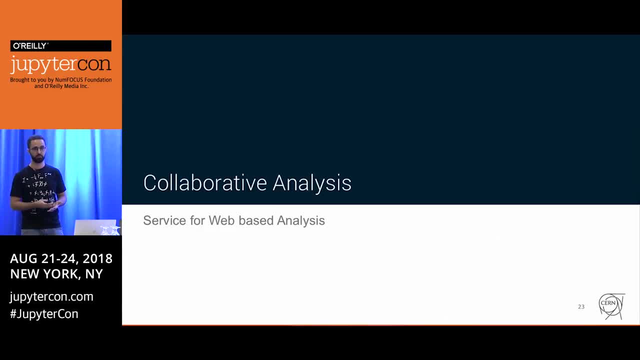 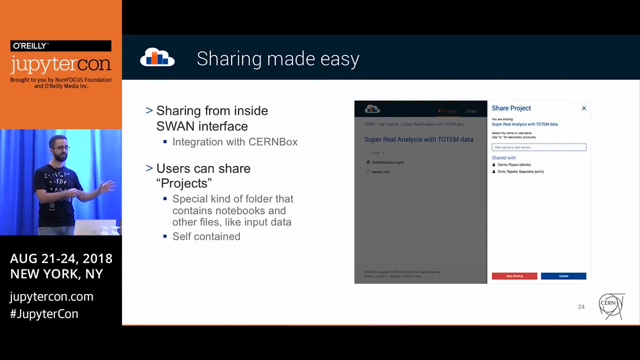 very important. at CERN, no one works alone, so they constantly need to share their work with a supervisor, with a colleague, with someone outside of CERN, and so it was very important for us, the sharing functionality, and so we decided to bring it inside the Jupyter interface. and now 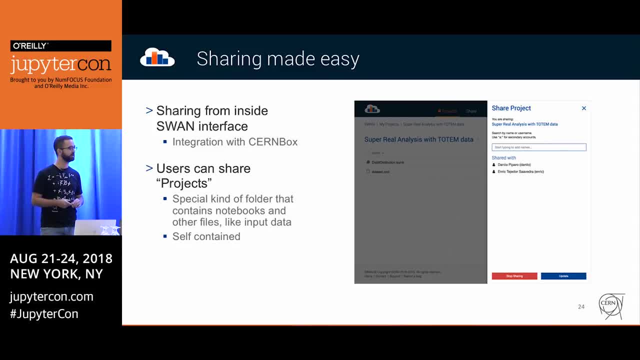 the users don't need to go and switch between certain box and and so on, because they can share right from within the interface. and when we did this we thought usually users share their notebooks, of course, but they only. they also share input data. they can share some pictures, whatever they need for the 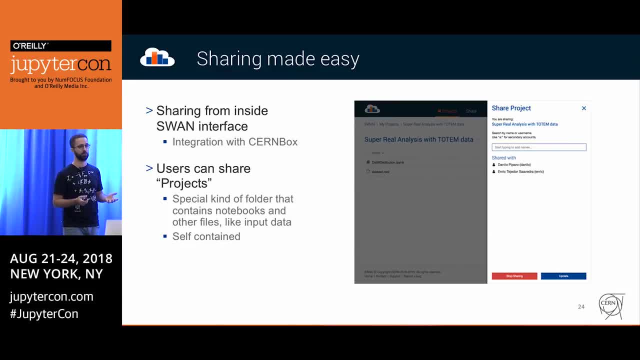 project, and so we decided to create what we call a project, and a project is more or less like it's a special kind of folder, let's say like this, and it should be self-contained. and this is the single best way to get people to work with Jupyter, if we can. 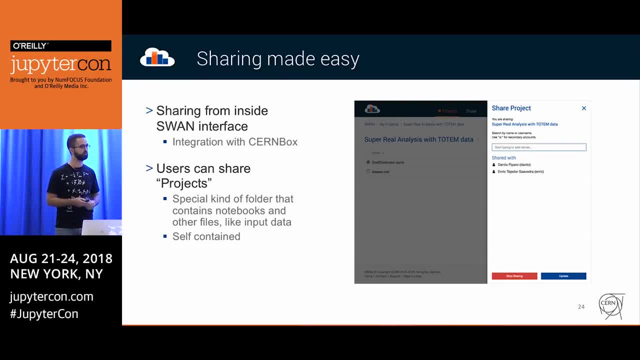 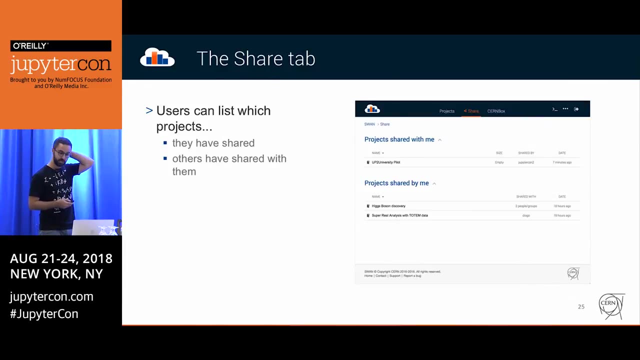 unit of sharing that you can share from swan. so when you share something from swan, it needs to be inside a project. it's a simple way of looking at this and it it simplifies the process for our researchers. and, of course, when you share something with someone, you can see what others share with you. you can even open. 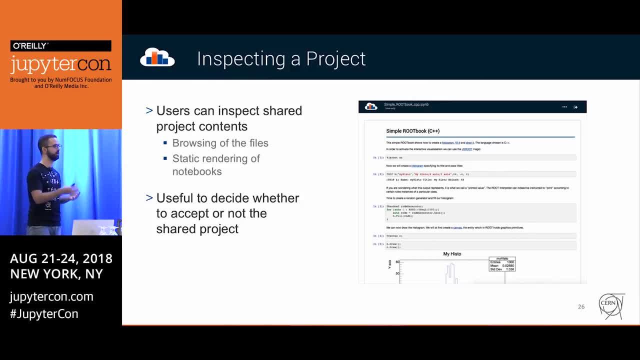 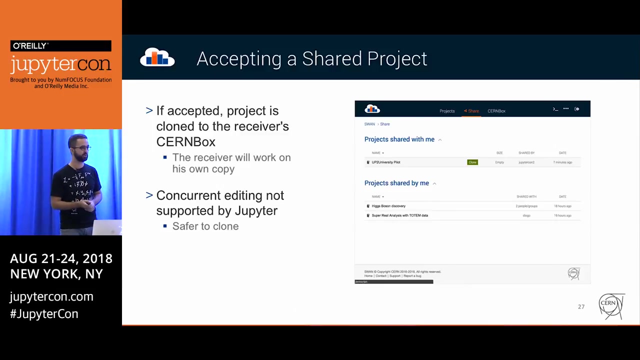 the share projects and look inside. look what files are there. you can see notebooks in read-only mode, and the idea here is that you know what is inside so that you can decide: does this make sense to me, can I work with this or do I need to work with this? and this is because we provide users the ability to clone. 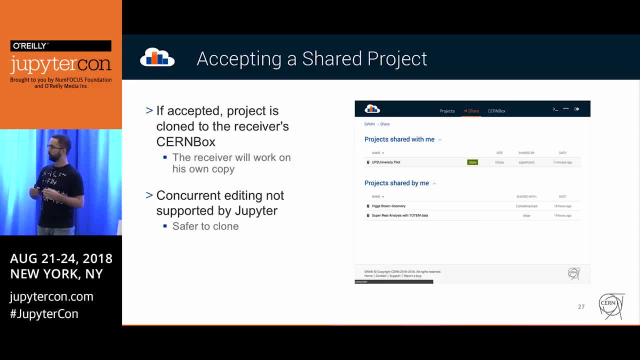 projects into their own user space. so you can see that we have the ability to clone projects into their own user space. so what they do is that they get a copy of this project inside their own certain box, and we we do this for a sing, a simple reason: currently Jupiter doesn't. 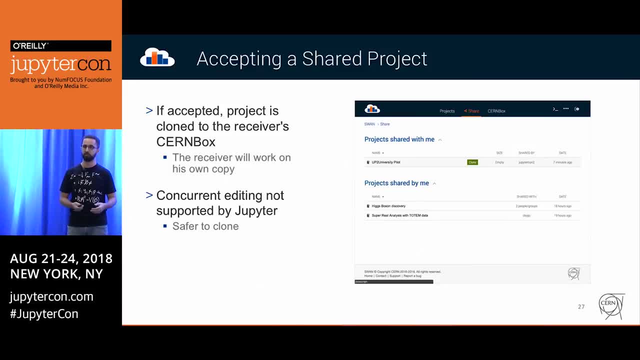 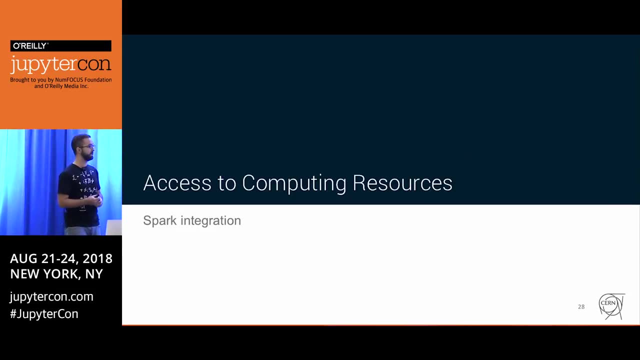 allow concurrent editing, so it's much safer for us to provide this functionality through a cloning mechanism than by sharing the folder with two people at the same time. and again, once we provided this, our users liked it. yes, yes, yes, okay, so we provided these new functionalities and, of course, our users wanted more in. 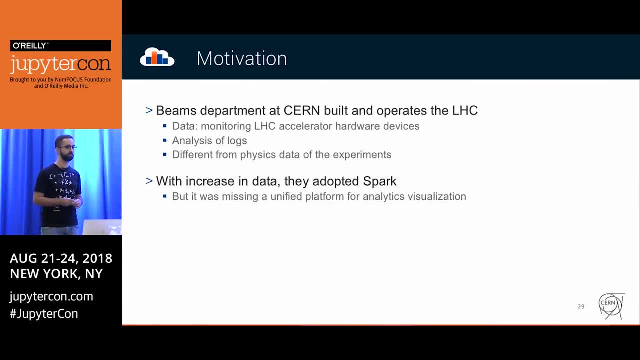 particular department at CERN, which is the PIMS department. they are the ones that build the ALHC and they are the ones that today operate this machine, and what they do is that they collect logging information from all the devices across ALHC. and this is an interesting case, because we're no longer 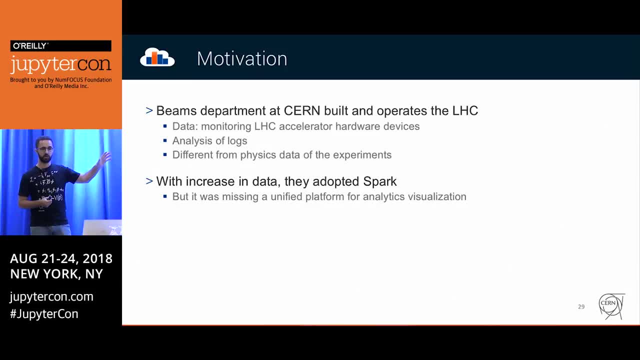 talking about physics data, the physics data that come out of the LHC, but all of these logs that come out of the the machine, and they decided to adopt Spark to process all of this data, but they were missing a unified platform to do the analysis, and so they came to us. they asked us if we could. 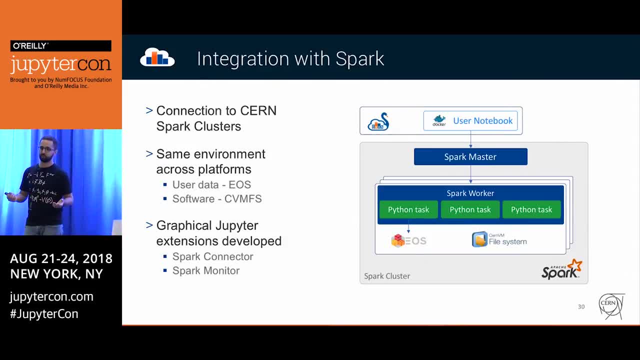 provide such a platform, and so we decided to integrate Spark inside SWAN, so now you can access the, the CERN cluster that we have, right from within SWAN, and a very important thing here is that, thanks to EOS and thanks to CVMFS, you have the exact same. 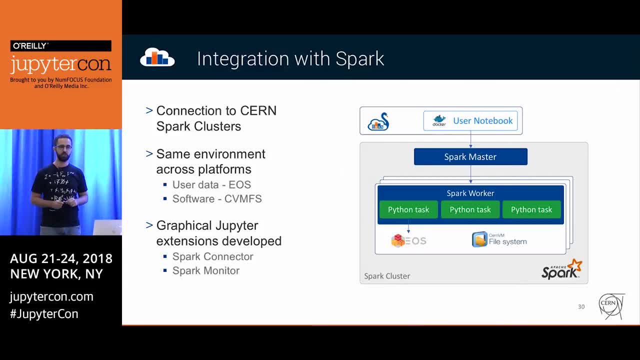 environment, both locally and in the cluster. so if you have, if you are working in your notebook, you can try it locally and you know that it will run in in the in the Spark cluster because it's the exact same environment, even though these are completely decoupled. but, as you can imagine, usually these jobs take 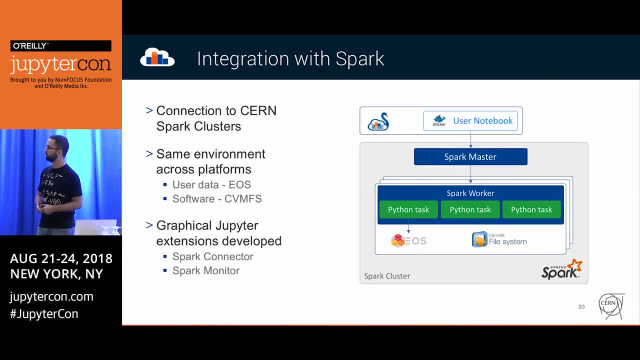 a long time to to finish, to produce results, and this defeats the purpose of interactivity. so we had to provide some tools that would give the users this interactivity that is common with Jupyter, and so we developed two extensions for this. the first one is the Spark connector, so you 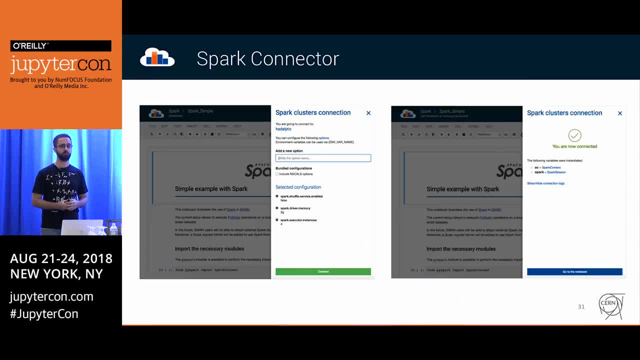 just need to click a button and you can configure all of your connection. you can set all of the properties that you need for Spark. you hit connect and You get some animation with with the logs that are coming out of the cluster, and then you are connected. You are ready to go. We export this into the notebook. 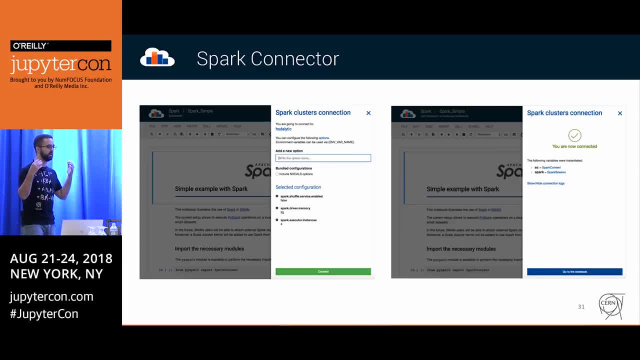 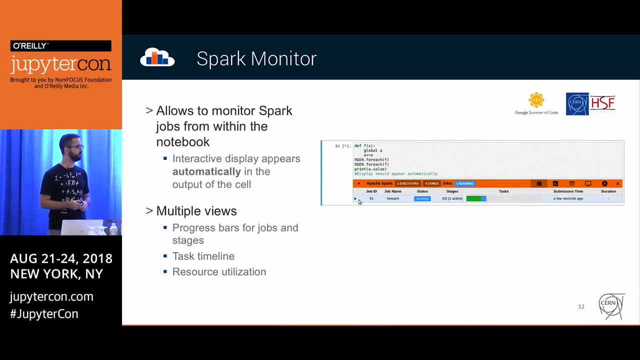 we export spark into the notebook, and so you can start writing your analysis without doing anything else. and When you do so, when you write your analysis and you submit the analysis to the cluster, You get this. This is a monitoring tool that appears automatically below the cell that you run, and 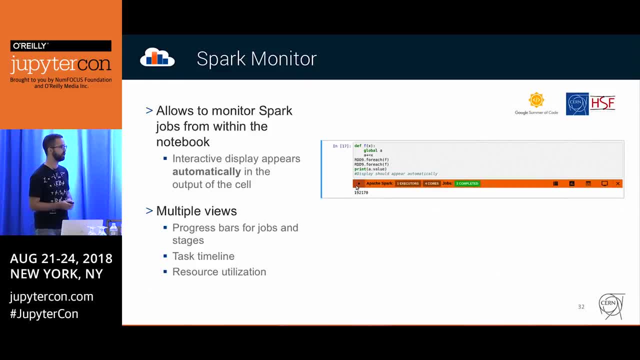 it allows you to see all the progress bars for the jobs that were created, and you can even see the task timeline and You can see the resources that we are using. and this last one is very important because, By looking into this, you can see if you are taking advantage or not of all the resources that were allocated to you. 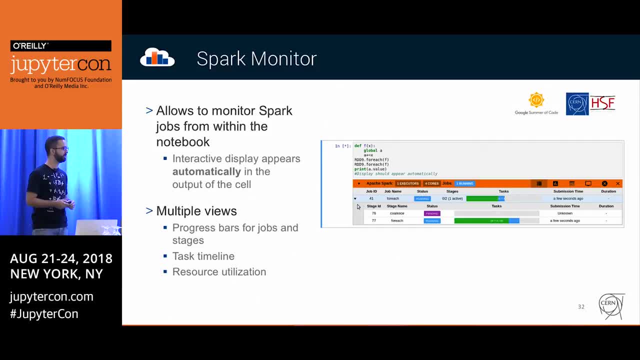 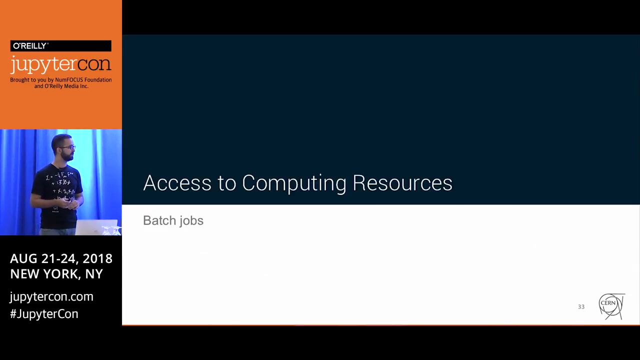 and An interesting thing of this is that this became The. it started as a Google Summer of Code project at CERN. We are an umbrella organization of g-soc and This is one of the many successful projects that we have each year, So successful, actually, that we decided to. 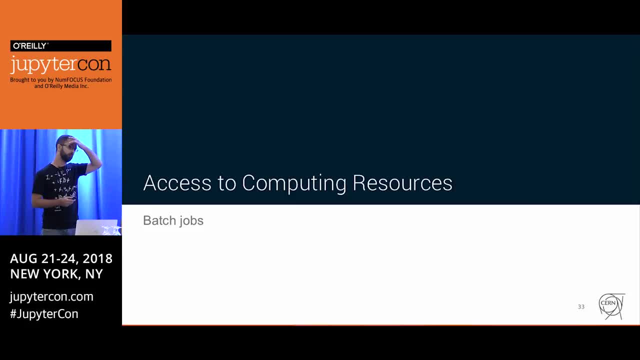 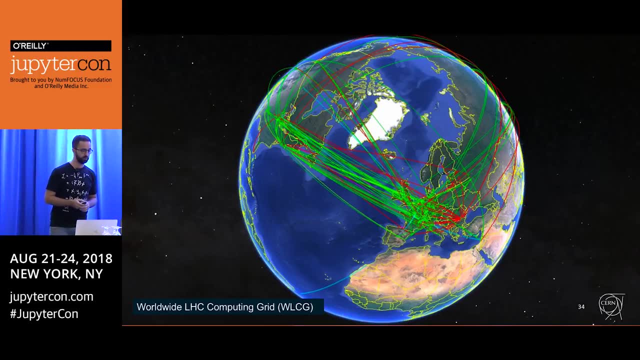 Create something similar this year, And so we thought about providing access to our batch servers. We have what we call the WLCG. This is the worldwide LHC computing grid. It's a worldwide grid that gives enormous amounts of storage and processing power, and 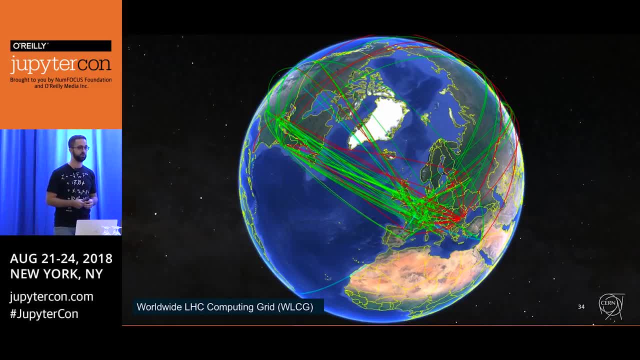 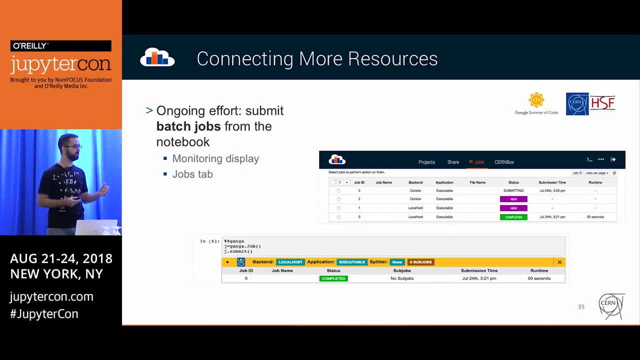 Our users are used to to submit jobs here, So it made perfect sense that we allowed them to submit their jobs from Swan and Just like they submit jobs to spark. and so this year again, as a g-soc project, we started building the integration of of batch inside. 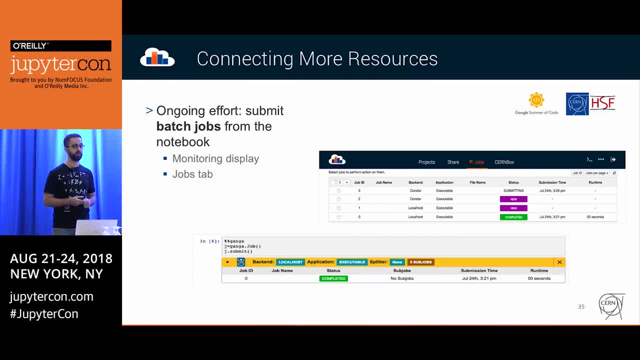 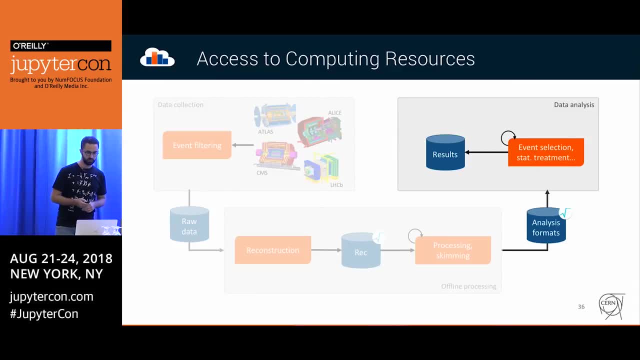 the, the Jupiter interface, and we did the same thing as park and we created some monitoring tools for you to see what is happening in the background. and If you look again at the pipeline that I already showed you, you can imagine that we are with this new high luminosity LHC. it will be very important for us to provide. 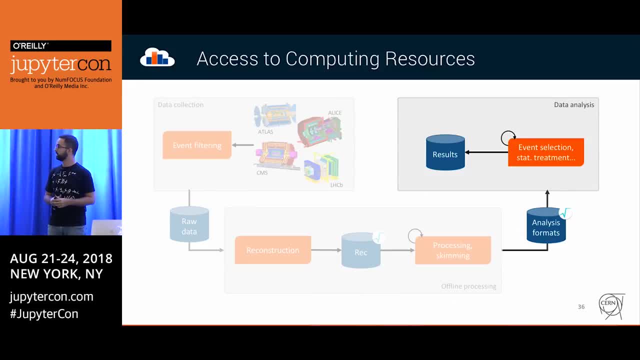 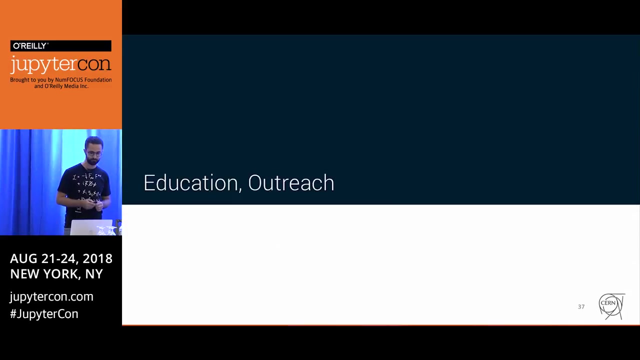 access to these enormous resources because they will need them to to provide the analysis that they do, but it also means that we can go a bit back in the pipeline and use one for the, the processing stage that we have, the stage where the researchers produce the analysis data sets- another thing that I 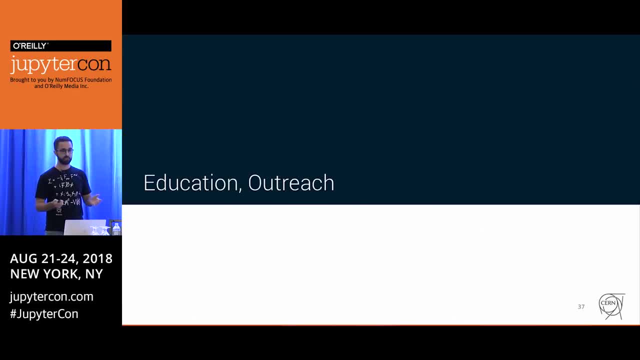 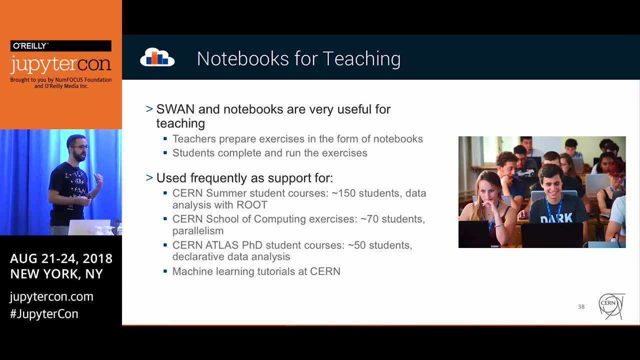 would like to talk is education. it's part of CERN's mission education, and we have a lot of programs each year. we just had in the last three months our summer students. we have them every year at CERN, but we also have tutorials all year both. 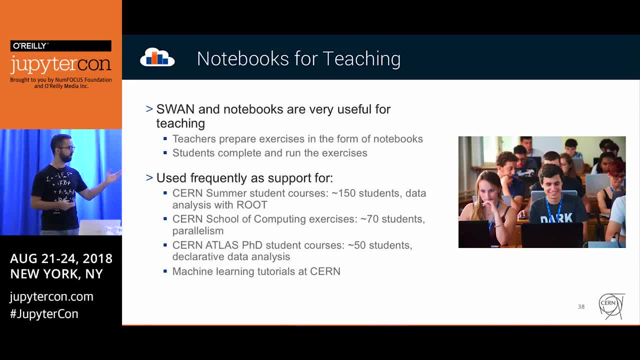 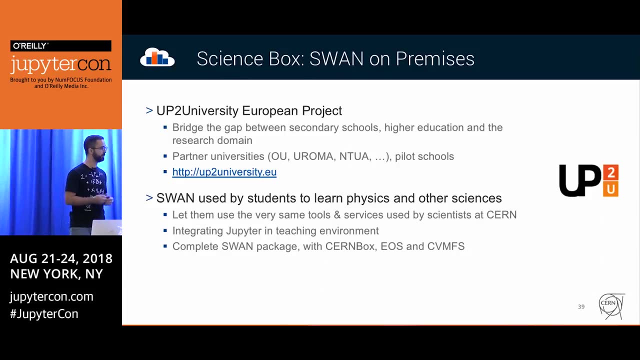 at CERN and spread across the world. we have a lot of PhD students that work at CERN and, as you can imagine, Jupiter is such a powerful tool for this that we decide to adopt Jupiter extensively for these activities. and we are even going a bit further and we have an European project. 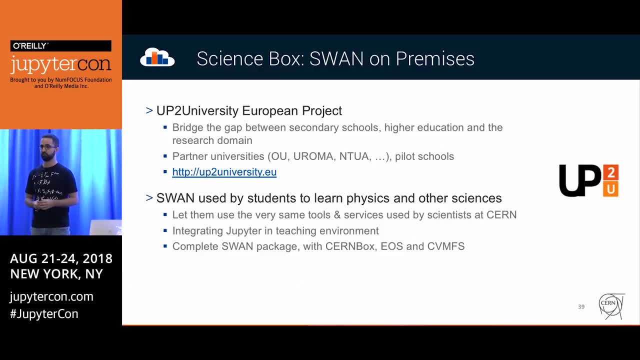 European funded project that is called up to University, and the idea of this project is to bridge the gap between higher education and University. so we aim to bring the tools that we provide researchers and to university students back to higher education for the students to start learning with those. 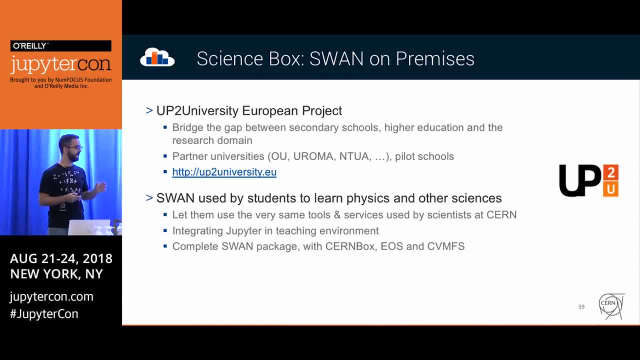 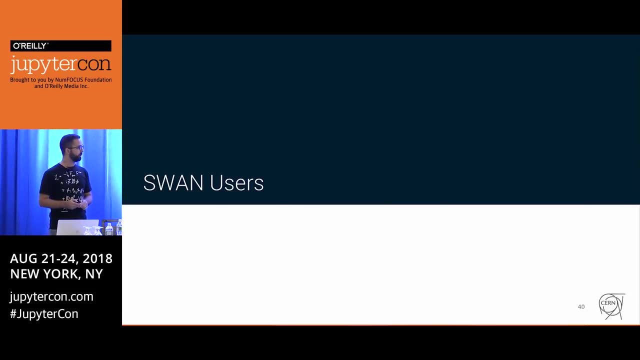 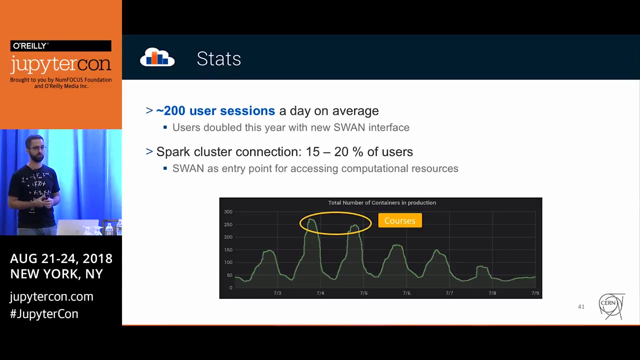 tools, and when I mention, when I say swan, it's the full swan. so all the software packages that the researchers have access to- EO, CVMFS- everything comes along. just a brief mention about our users. we have around 200 daily users. it more or less double since we deployed the new interface. we're also seeing 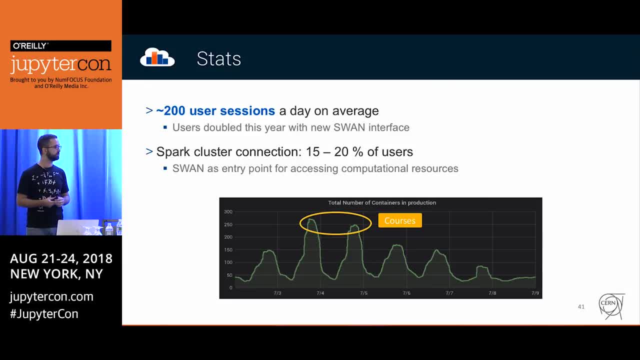 growing numbers with when we start deploying spark, which was a couple of months ago- and we also see an enormous increase in in the usage when we have courses and tutorials. many times we don't even know that's something that we're going to be able to do in the future, so we're going to have to. 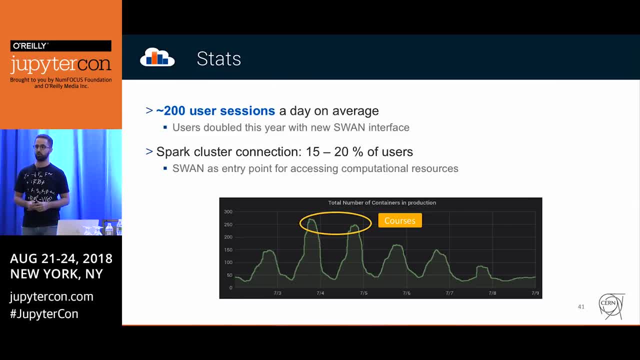 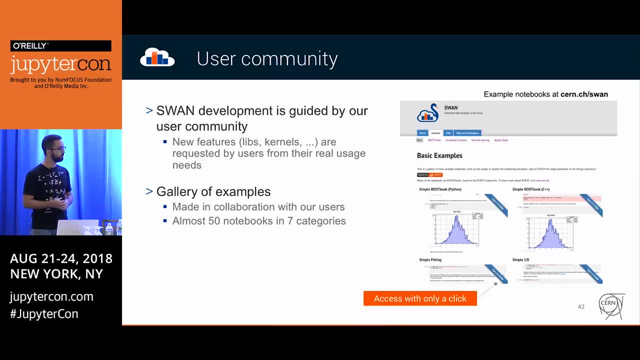 someone plan a tutorial that uses swan. but when we look at the numbers, we understand what is happening and our community is very important to us, because it's this community that is helping us shape what swan is. I mentioned the example of the beams apartments, but there are others and they usually come. 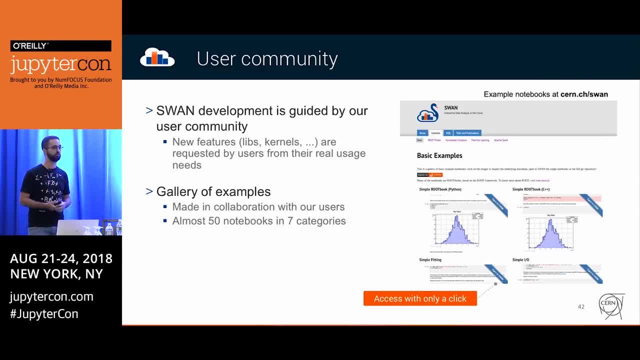 to us. they ask us for functionality. we work with them to to make, to integrate these functionalities inside swan and in the end we have the habit of creating notebooks that exemplify how you can use these functionalities. so if you go to CERN, dot C, dot CH, slash swan, you can see almost 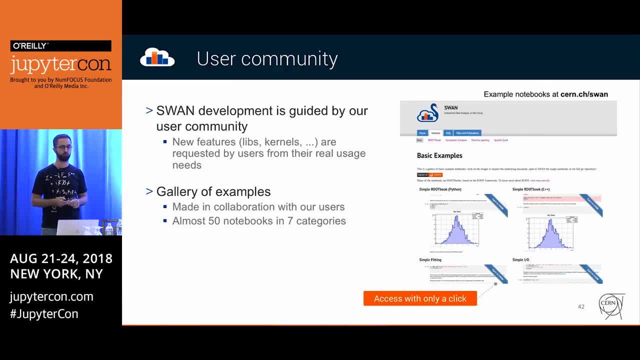 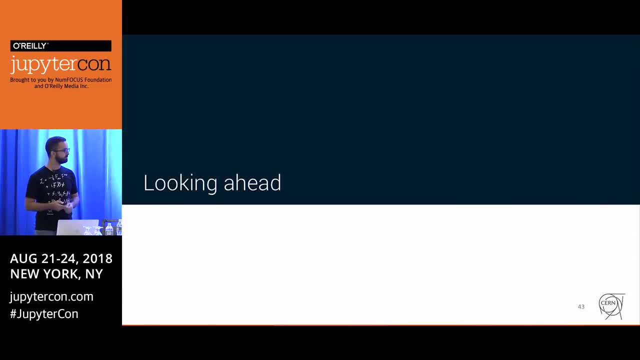 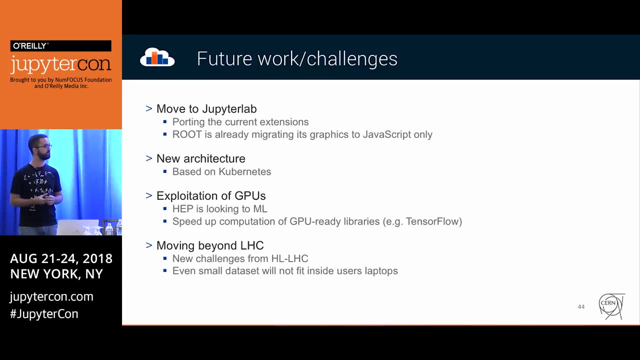 50 notebooks that exemplify how to use one, and most of them with related to physics. but let's look ahead, and this is what we're really looking at right now, so what we're planning to do with the platform. the first thing is to move to. 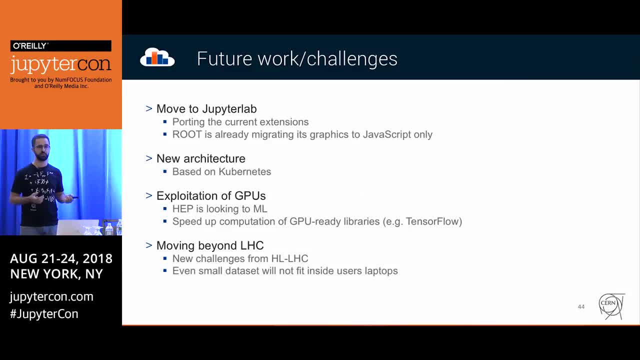 Jupyter lab. as you can imagine, many of our users need more powerful tools than what traditional notebook can provide, and we think this will be a way for to attract these users that don't see swan as a useful tool for them. and, of course, this means that we will have to port all of our extensions and 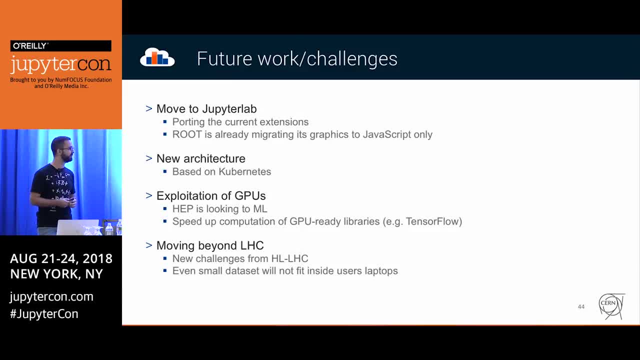 but it's part of the job, right. and then, of course, we also want to investigate a new architecture for the service. we are studying the adoption of kubernetes. we also studying the usage of GPUs, because the the HEP community is now looking more and more to machine learning and we need to provide them GPUs, because these are. 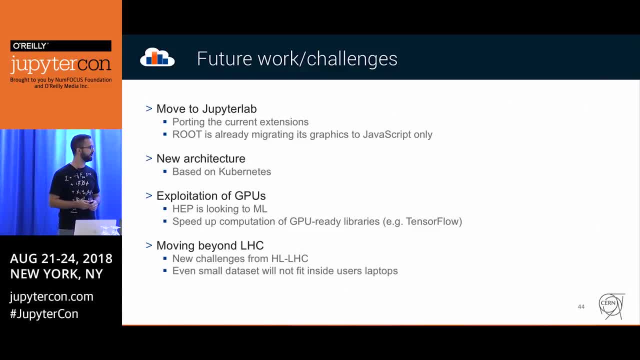 the what brings some speed to their analysis. and lastly- I already mentioned this- we are moving ahead with LHC. we are bringing the new high luminosity and this brings a lot of new challenges that we need to to solve, and I think swan is getting ready for. 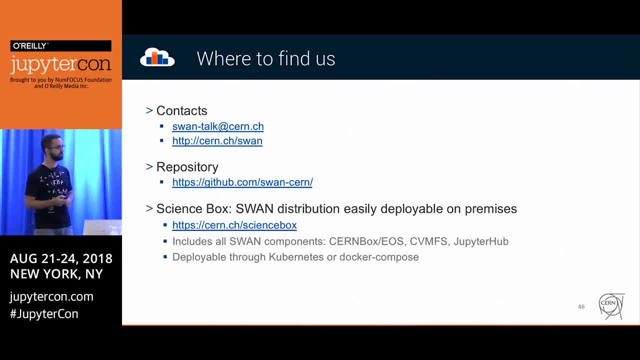 for them. if you want to find us, these are our contacts, our email, our website. most of our code is public- not all of it as of today, but, uh, we are working to to make this available, and we also have what we call science box. this is what we use in that European project. 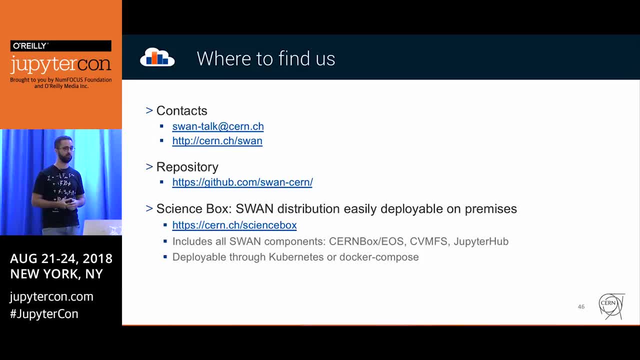 called up to you. so we containerize all of our, our services, and you can access and deploy them using kubernetes or docker compose in your own infrastructure or in your own computer to try it. but just a heads up here, new interface and functionalities. they are still not there. so this is a bit 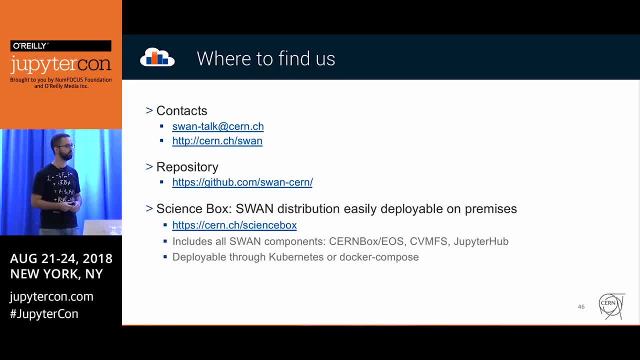 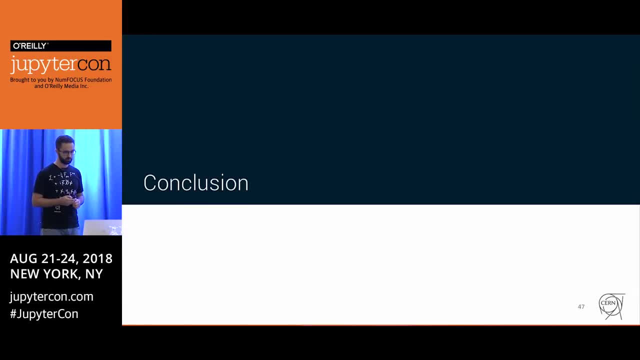 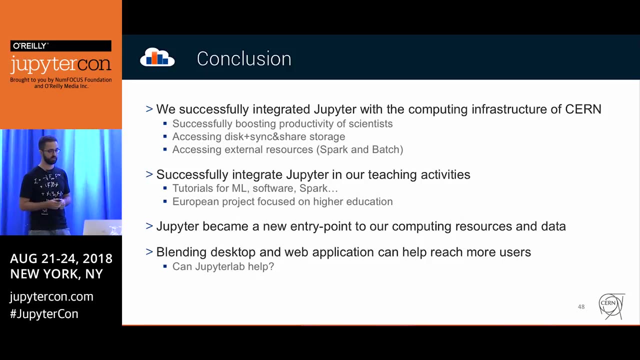 behind our production environment. we are working to to bring them into this containerized version, hopefully in the next months. just to finish, what I think you should take from this presentation is that we did a lot of integration with Jupyter. we are really providing Jupyter notebooks on top of our infrastructure. 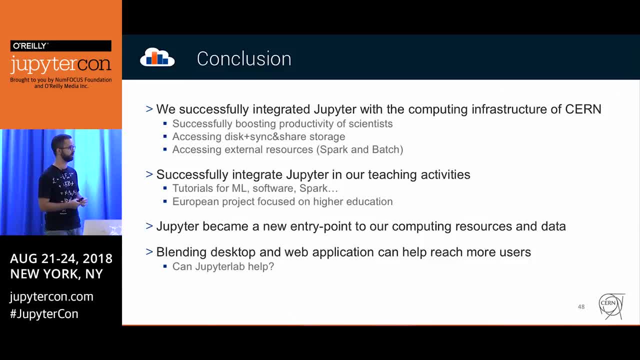 and by doing so we are boosting the productivity of some of our researchers and we're giving them access to disk sync storage software- everything without the need of configuration and installation. I also want you to remember that Jupyter is very important for us in education, and in the future we will be using Jupyter for all of our projects. 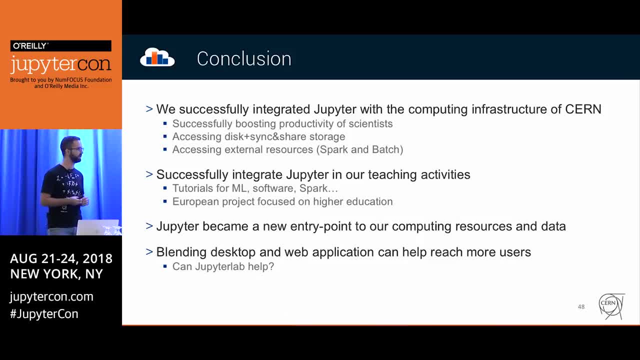 and we will continue to do so in future projects, and we will continue to do so in education. we have a lot of programs and we use it extensively, and something that summarizes all of this is that Jupyter is becoming an entry point for all of these massive resources that CERN has, so they have other entry points as of today. 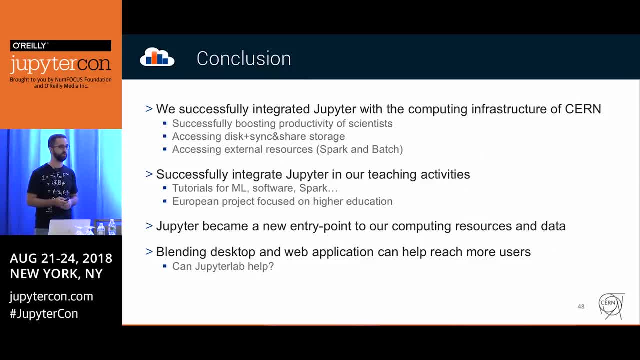 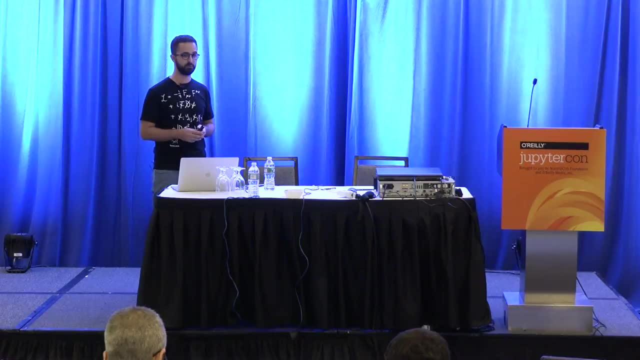 but Swan is becoming a very important entry point for this and, lastly, of One of it is to provide more powerful tools, and we think that JupyterLab might help, And so this ends my presentation. I think we still have time for some questions. 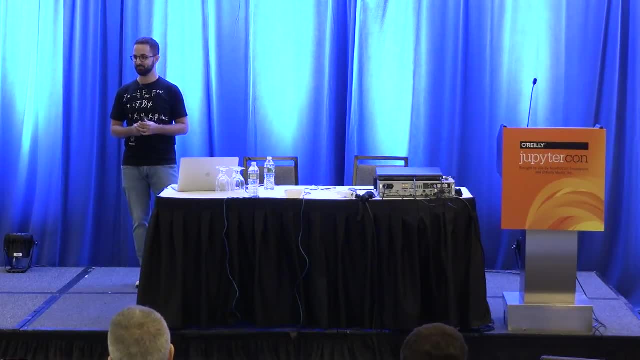 I hope you're not bored to death, Thank you, Thank you. So Root is mainly C++, but it has automatic bindings with Python, so you can also do your analysis in Python using Root, and that's how we integrate it. The kernel uses Python to connect to Root. 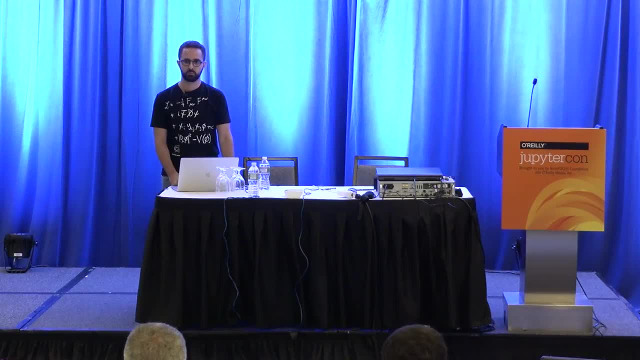 So, for example, if you have C++ with Python, it's just a question: do you think that you have multiple interfaces that you can find in the version that you want to use so you can develop something and not develop Python? and there's a lot of different ways to do. 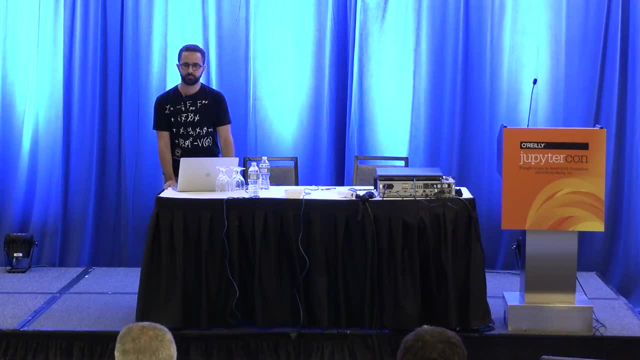 it in Python. Yeah, So how is that? Is there any kind of merging of the pictures that you can find in your mind As of today? it's a lot of work. It's a lot of work. It's a very simple service. so you share it, you clone it and, if you want to get back, 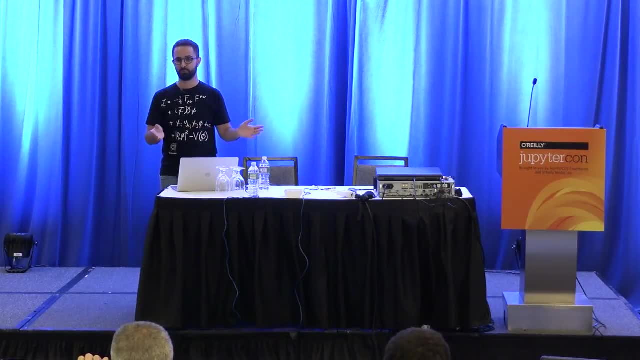 to the original owner. you need to share it again, So for now, we don't have any other way of doing things. Okay, So where is the Jupyter question Is the user type? you know the cache that I'd like to use in Python. 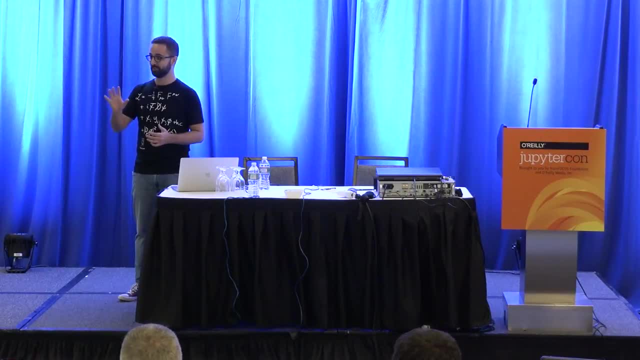 It's running inside the kernel in part. I'm sorry. It's running inside Docker container that we spawn. We have machines dedicated to swan, So they have they provide the compute power to. I'm not sure, but what I imagine is that they submit these batch jobs into the grid. 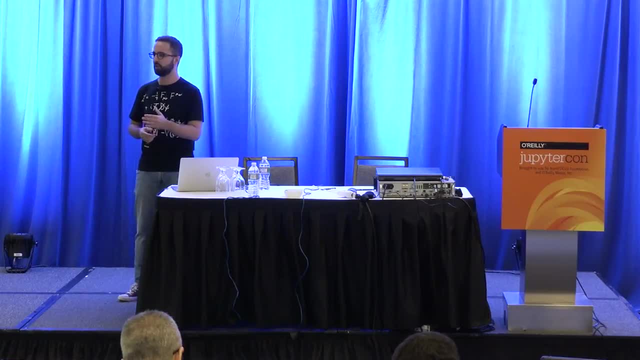 There, they can submit and do whatever they like. And actually, yes, we have what we call LX plus. It's a you can do, it's a terminal, you can do whatever you like, and it also provides computing power. So do you reuse it or use Spark? 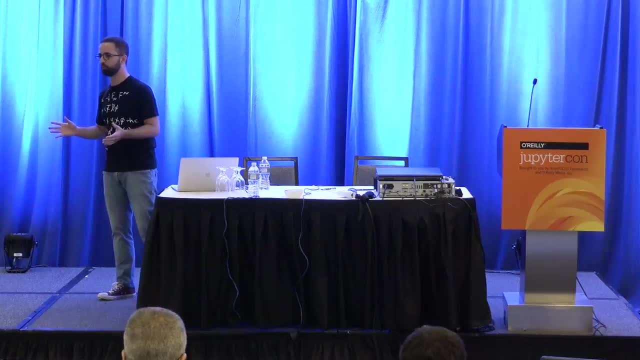 This is something new- Spark. So they are not used to use Spark. They are starting to use it now but, yes, they can use the command line to submit some Spark jobs And they use this LX plus that I mentioned. but now they're migrating into swan because 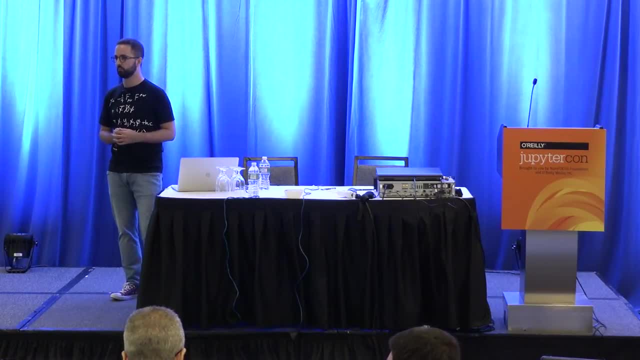 it's simple for them to use. So for our users, they use swan. so I was just wondering. I guess there are issues with running Jupyter on the computer. In our case, we do this because it's our service, it's our machines, we know we configure them. 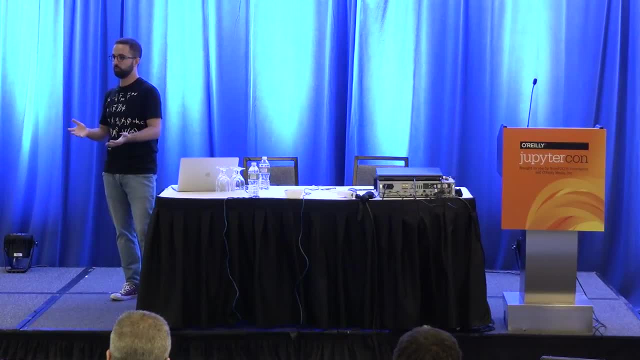 so we control this environment. If they want to use Jupyter, they can still use Jupyter, but not swan Swan is the service that we provide. Yes, We do that in the batch service. yes, and that's what we integrated into swan. 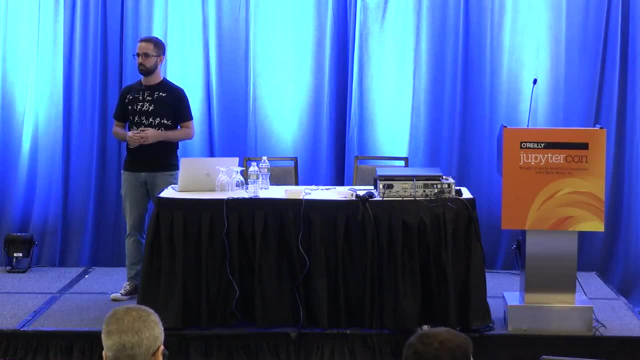 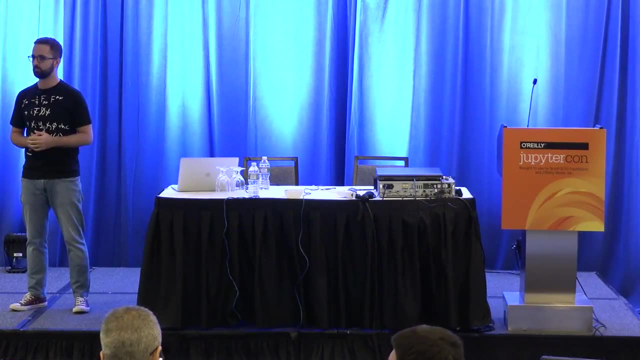 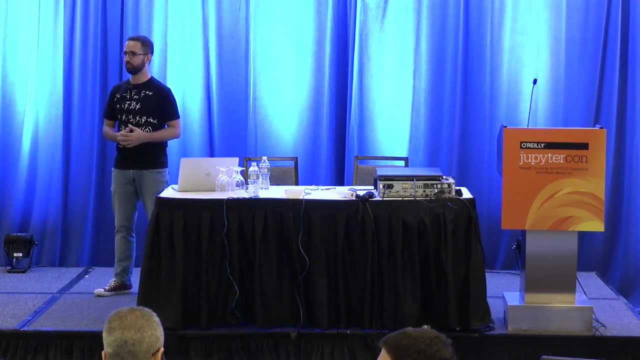 You submit your job and it gets scheduled. yes, Sorry, I'm, I assume, so I'm not an expert in this batch system, but I assume they can do it. yes, So everything that is produced in this batch jobs, it's written into EOS so you can just. 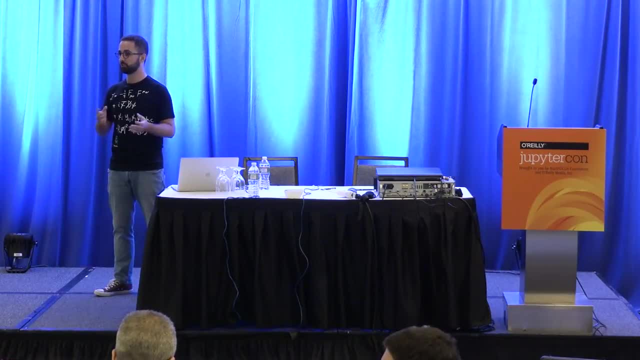 look at the logs that are produced there And actually that's a way users get their results. they look into the files created in EOS to see the results And we're trying to bridge this gap and make them available right in swan in the notebook. 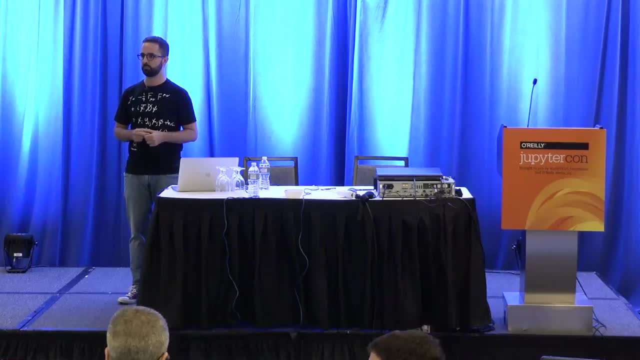 Yes, All right. So let's talk a little bit more about what your like as far as what you're going to be using for this. So, basically now, what we have with Kubernetes is this, dockerized, this version that we have. 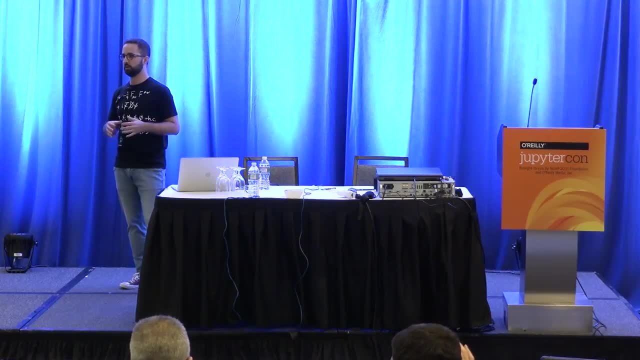 this science box version- and yes, we have. it's a way of spawning user sessions. We have containers for each of these components And we have you can create, for example in our pilot, for up to you have two machines. 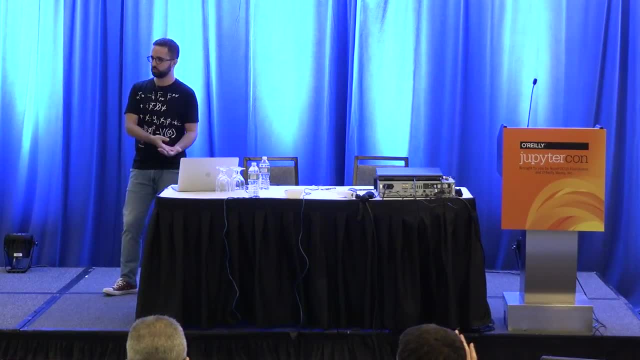 where you can start your session. This is how it is today, but we are still investigating what we should do next, Something that we thought was to deploy only the kernel itself in externally and access it, but it's still not set in stone as of today. 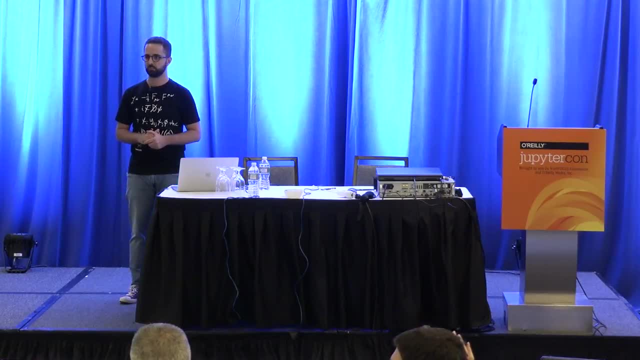 Yes, Okay. So, as you can imagine, CERN has massive resources, so of course we provide centrally, So every machine that we run, we have an orchestration system which is Puppet, and we deploy these services using Puppet. 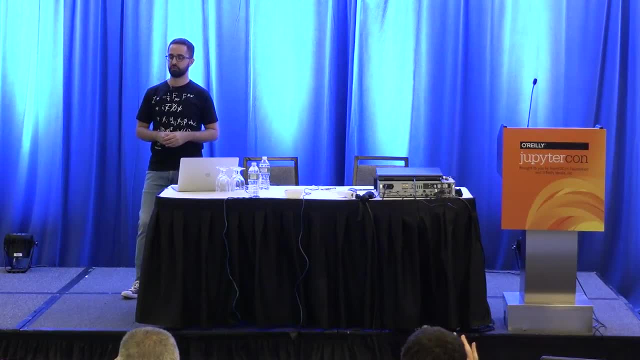 And by doing so, all of this functionality comes along, because it's mandatory for services that run at CERN. So that's how we get all of this information And of course, we have a system where you can set maintenance scales- Everything. 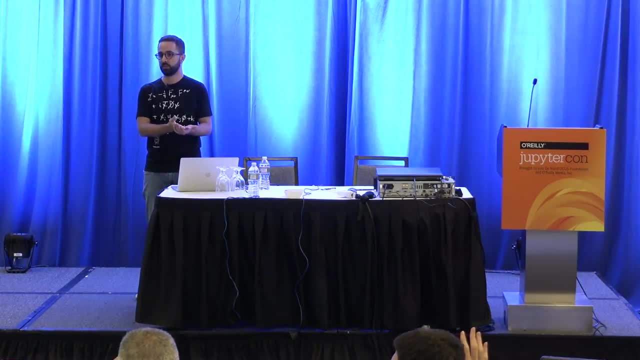 So it's a ticketing service. So when our users create a ticket because something is not working, there is someone that will redirect them and show them: this is downtime, this was programmed, so everything is fine. You just need to use something else as of. yeah. 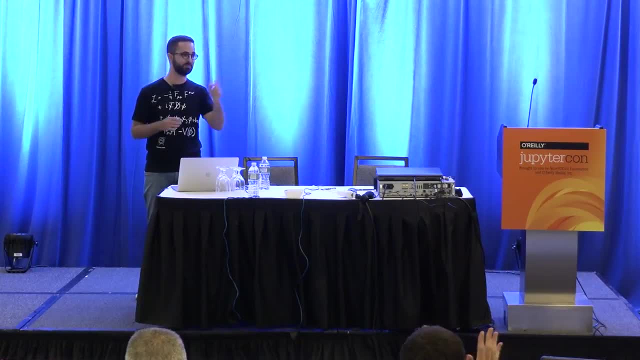 So, yeah, maybe there- Yes, that's actually- we had a visit of a person from Jupiter team. They came to CERN and that was the first question that she made me: Don't you use Git for this? And the answer is no. 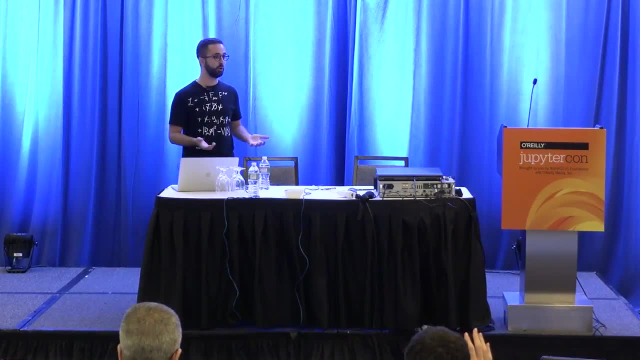 And actually many of our users don't even know what Git is, And also we don't have any tool that allows them to do this in an easy way. Of course they can use it. Jupiter provides a terminal, so they can, of course, use it to do it. 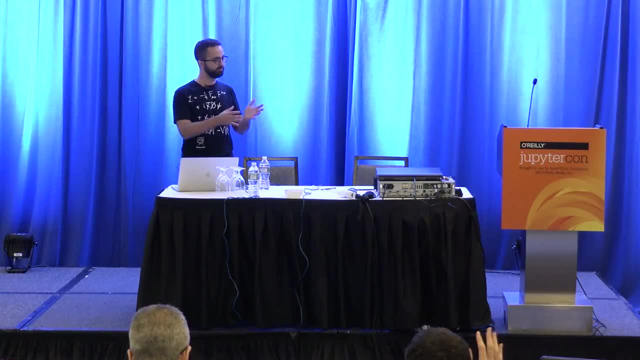 But we don't provide a graphical way of doing it. But that's one of the features that we are looking And that's why I say that JupyterLab provides such a more powerful environment, because all of these tools are coming along. It enriches all of the experience for the users. Yes.